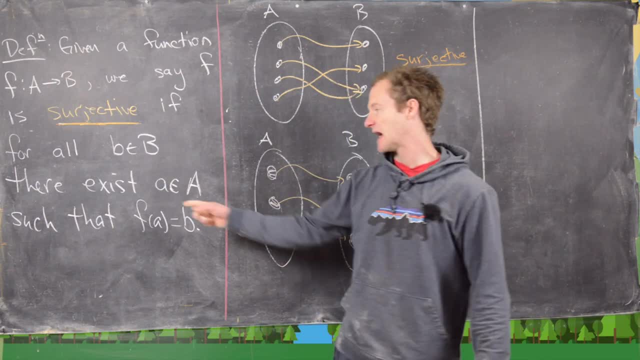 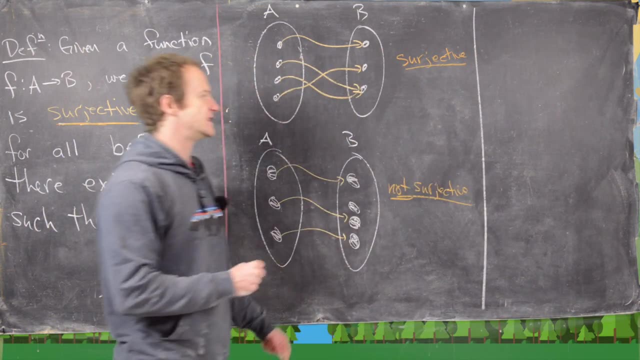 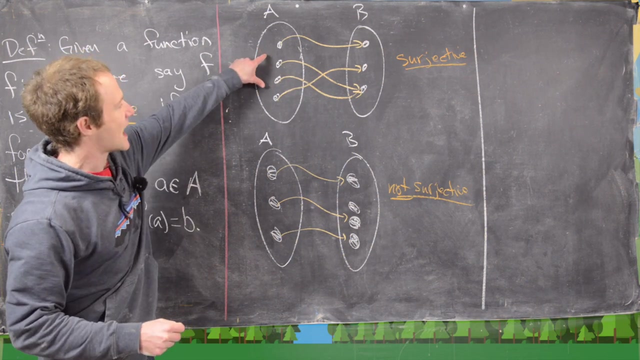 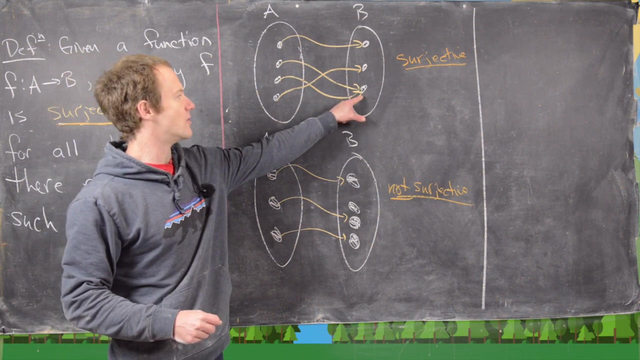 In other words, every element of the codomain has an element in the domain which is mapped to that element. So, generally, the first thing that you look at when you see these are these little picture diagrams. So here's a picture diagram for a surjective function. So notice, we have four elements in the domain and three elements in the codomain, but every element in the codomain is mapped onto by an element in the domain. 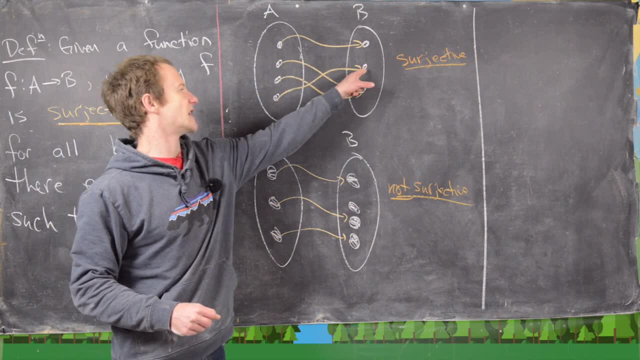 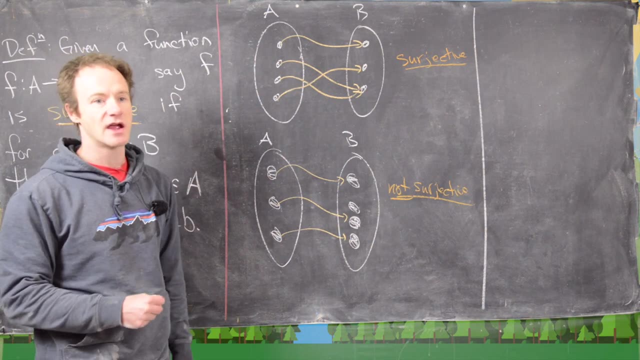 So this one is mapped onto by the first one, this second one by this one down here, and then this third one is mapped onto by two of these guys in the domain, And that's okay, you just have to be mapped on by at least one. 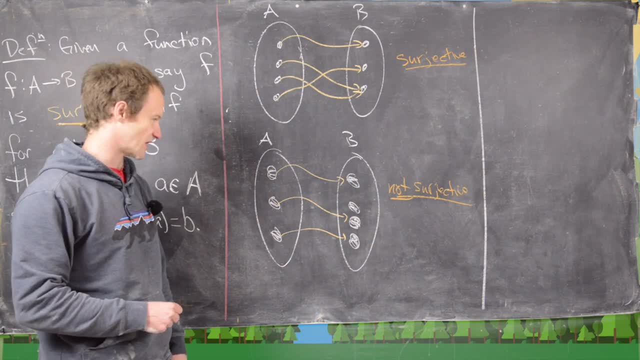 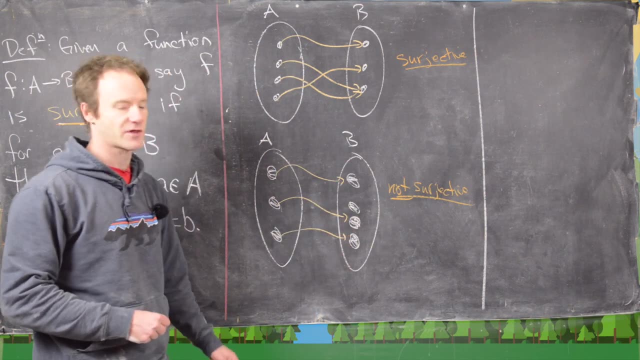 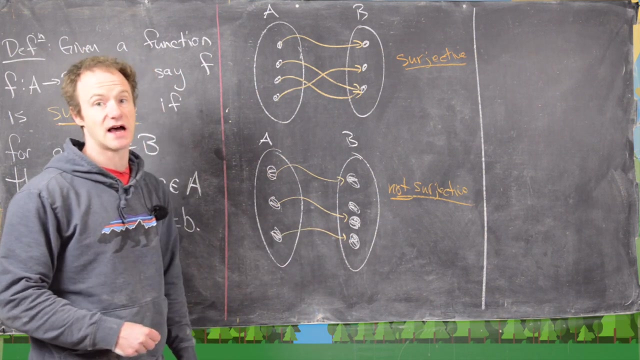 But then the second example down here is not surjective, because notice, this second guy in the codomain is missed. So this first, third and fourth member of the codomain is mapped onto by something over here in the domain, but this second guy is not mapped onto. 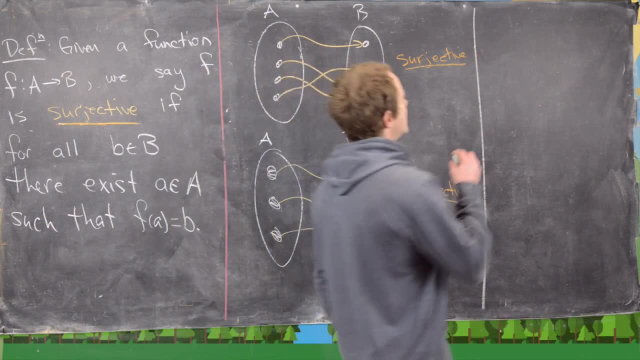 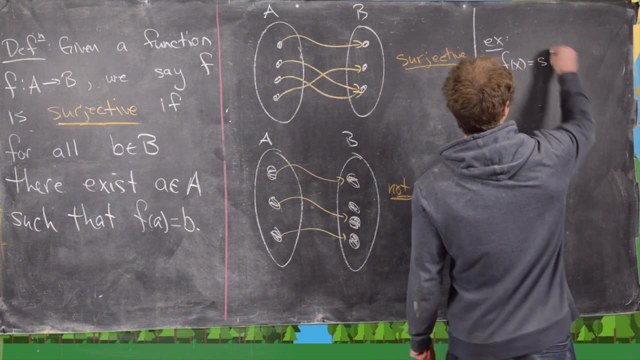 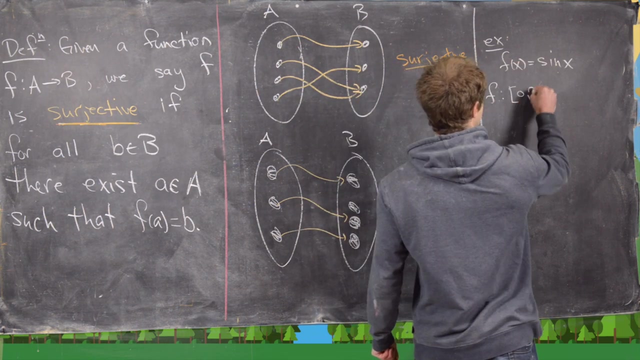 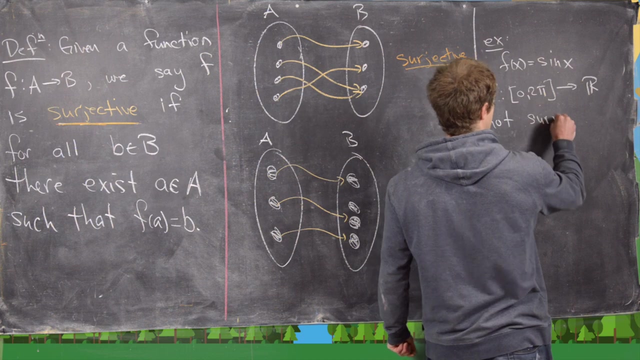 So now we could see some examples from calculus, and maybe one of which would be: if we consider the function F of X equals sine of X. And now if we consider this as a function from the interval zero to two, pi to the real numbers, this is not surjective. 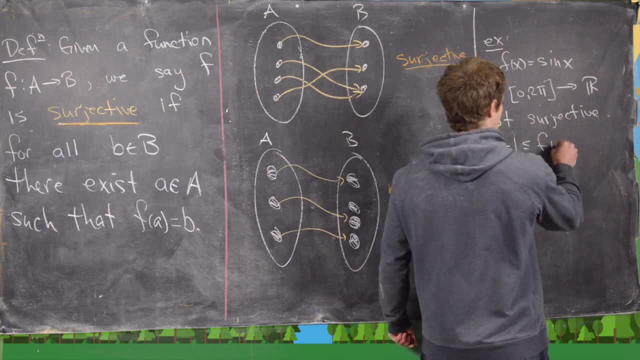 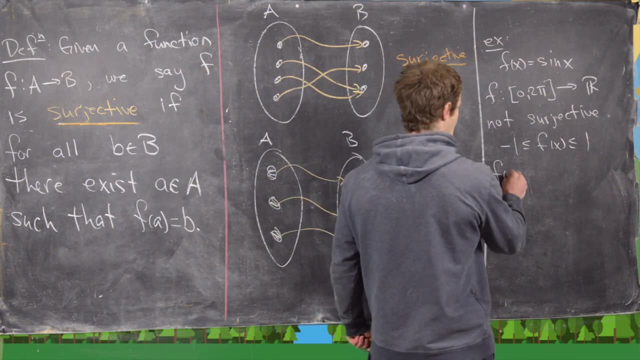 And we know that because F of X is always between negative one and one, And so, for example, F of X is not equal to two, And so, for example, F of X is not equal to two, And so, for example, F of X is not equal to two. 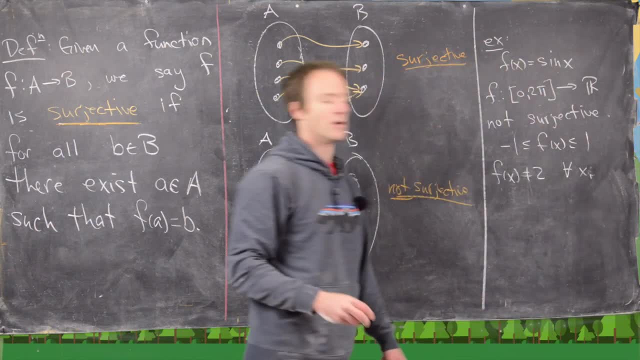 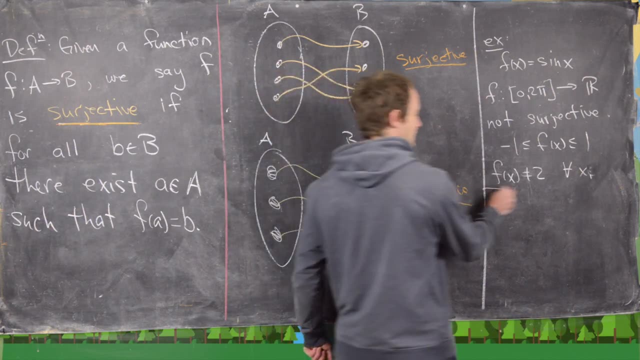 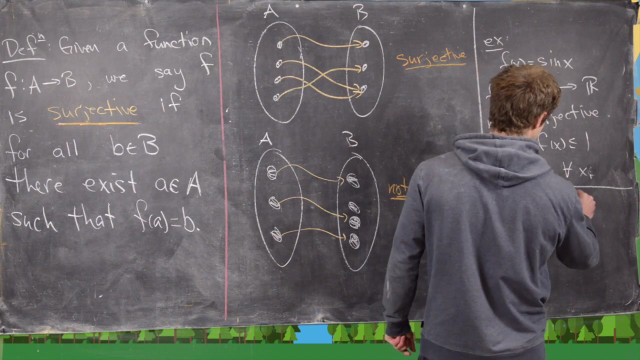 For all X. So in other words, two is an element of the codomain that is missed. But we can kinda hack this a little bit and instead view the same function. But now we are going from zero to two, pi to the interval negative one to one. 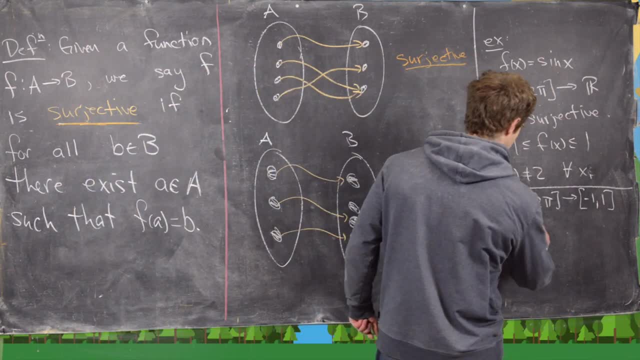 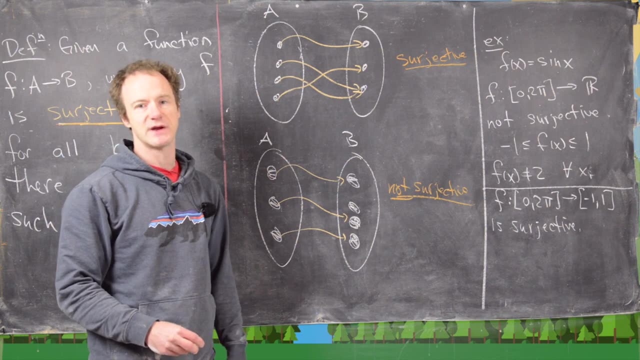 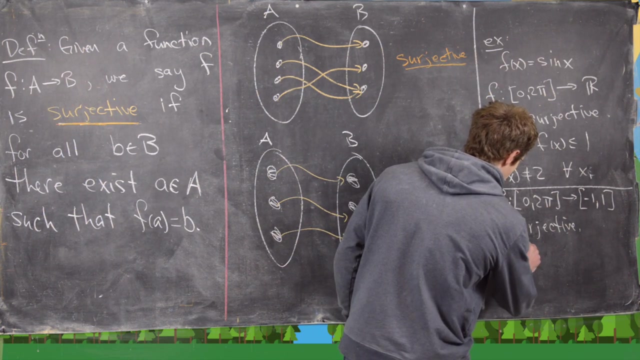 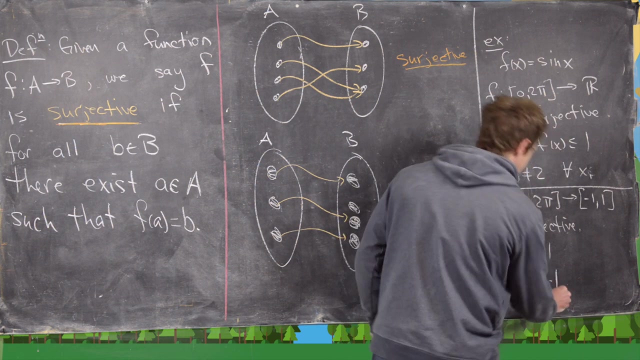 And now we know that this is surjective, Because f will achieve every number between negative 1 and 1.. And we can actually check that kind of carefully by noticing that sine of pi over 2 equals 1.. And then sine of 3 pi over 2 equals negative 1.. 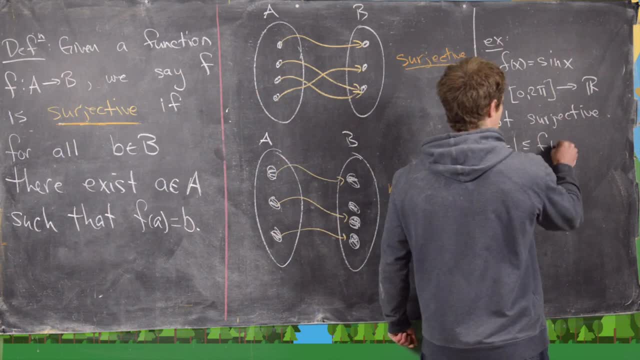 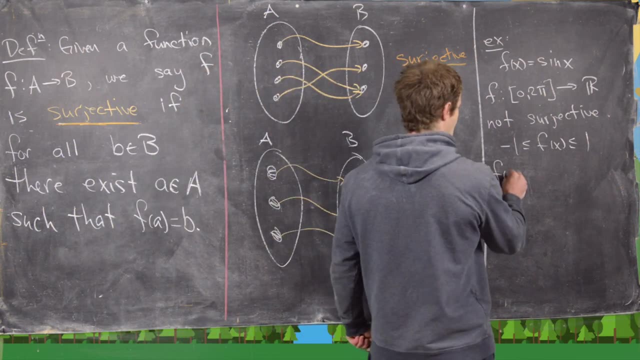 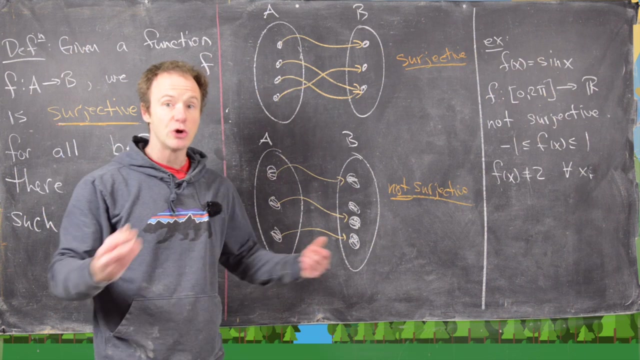 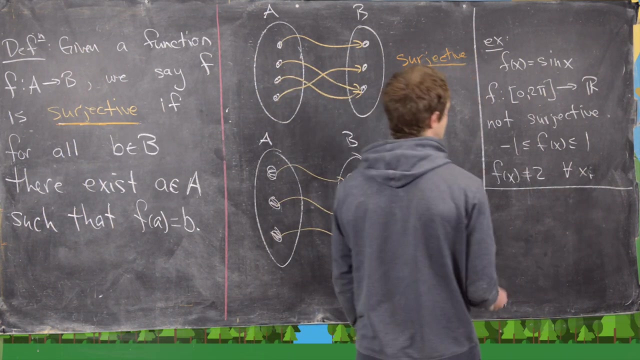 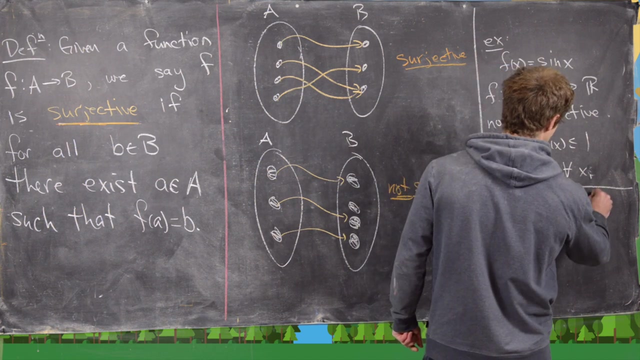 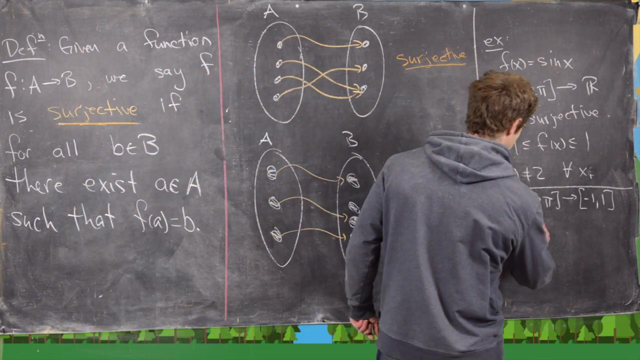 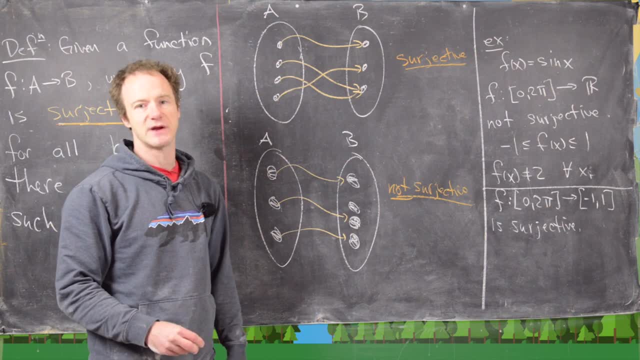 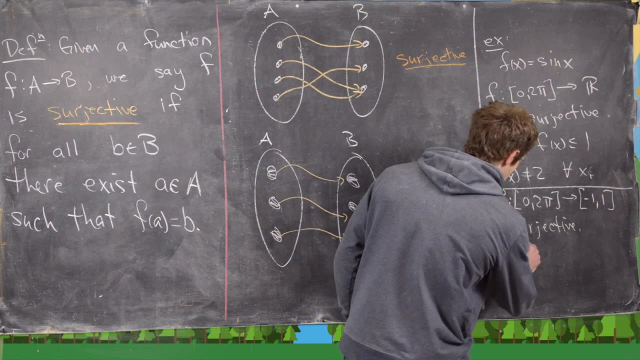 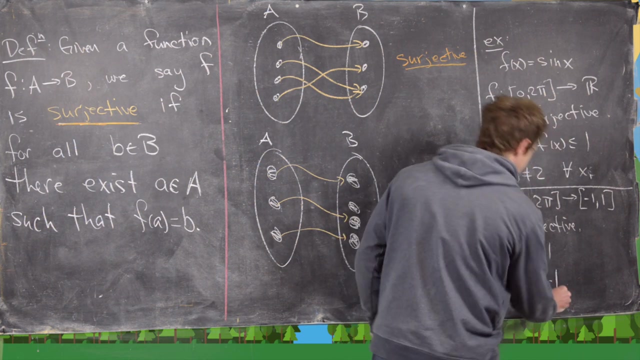 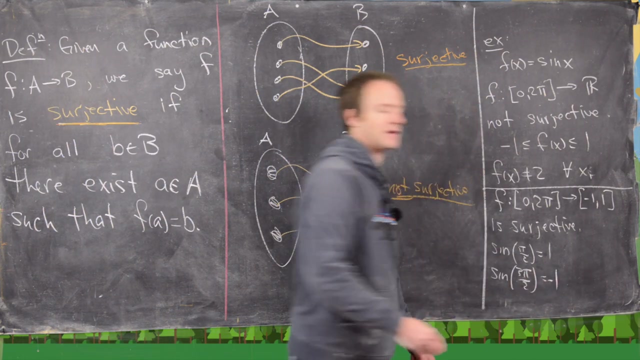 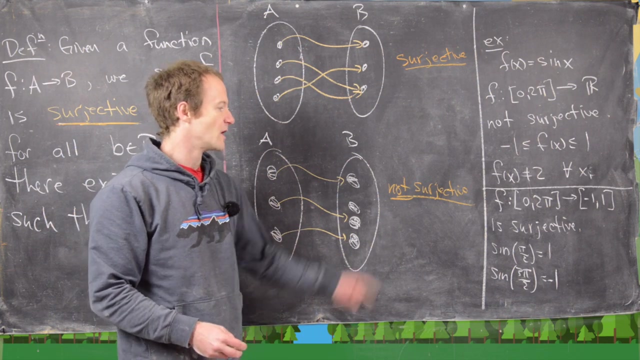 Because f will achieve every number between negative 1 and 1. And we can actually check that kind of carefully by noticing that sine of pi over 2 equals 1. And then sine of 3 pi over 2 equals negative 1. And so it achieves the largest number in the codomain and the smallest number in the codomain. But then using the fact that sine is continuous and the intermediate value theorem will show that it maps on to every element of the codomain. Okay, good. 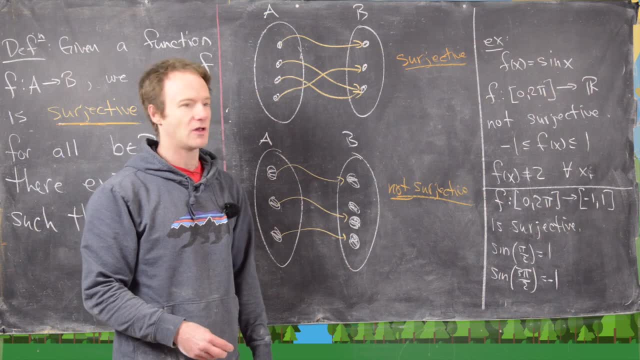 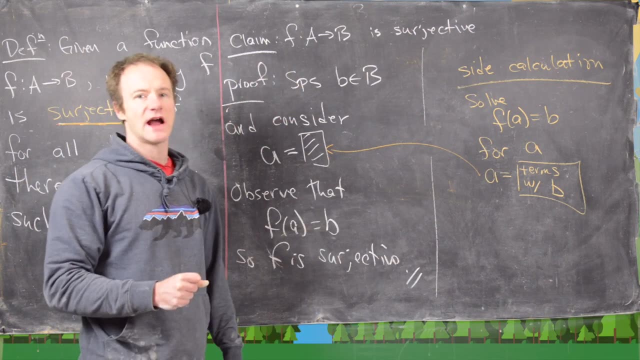 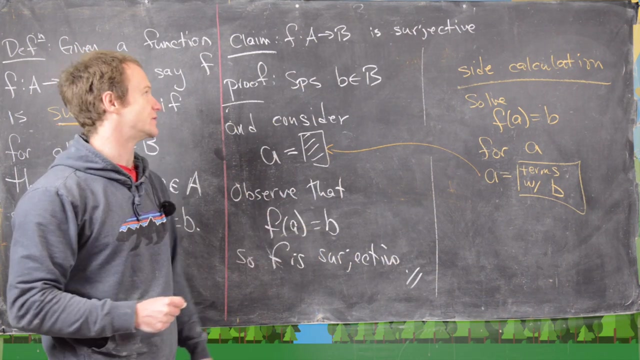 So I'm going to clean up the board and then we're going to look at an outline of a proof that a function is surjective. Okay, so let's look at the outline of a proof that some function is surjective. And it's really important that we look at this outline because there's a bit of a trick to it. And so... 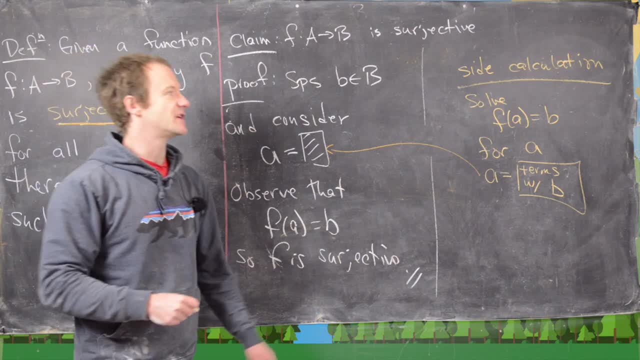 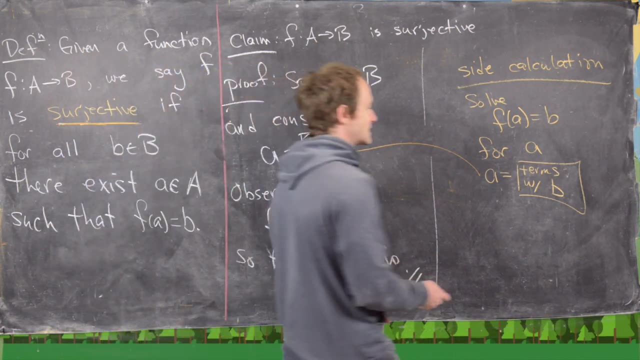 Again, our claim is that f is surjective. And notice, there's this really important side calculation. So this side calculation is not in the proof. And in fact, the side calculation in reverse will end up in the proof. And it will end up in the proof at the end. 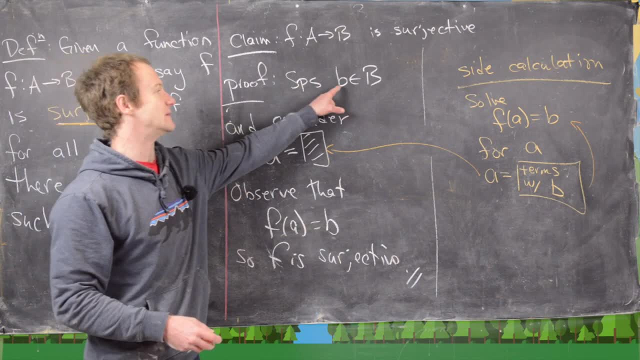 So let's look at the outline of the proof. So we suppose that b is in b. And so b is an arbitrary element. 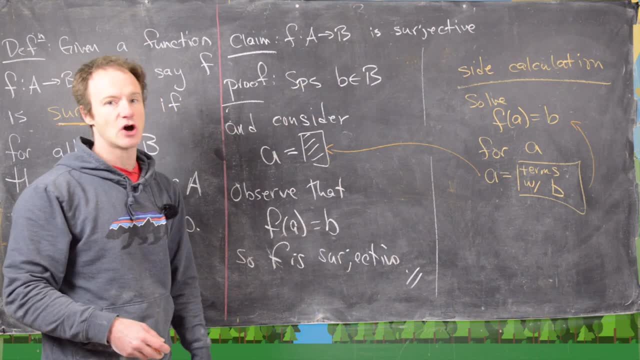 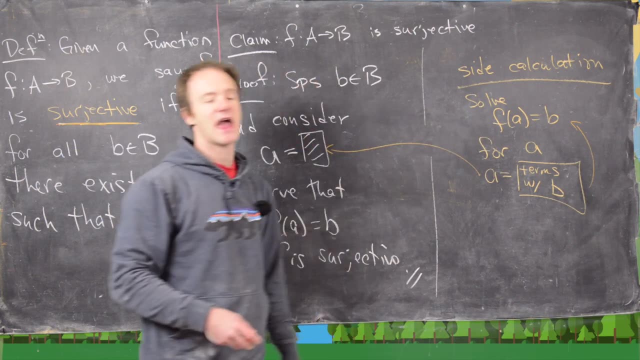 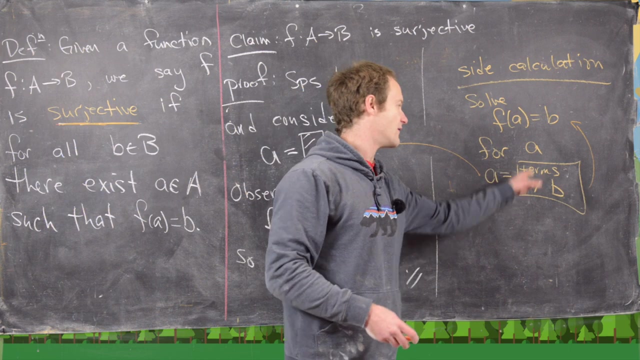 And remember, our goal is to find an element a from the domain that's mapped to the codomain. So we do that via this side calculation. So we solve the equation f of a equals b for a. And so what that will give us is a equals some sort of combination of terms with b. 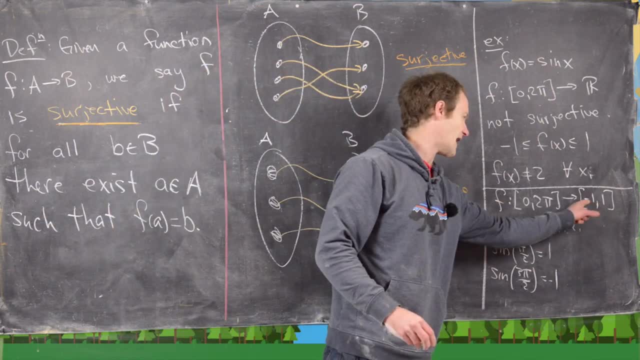 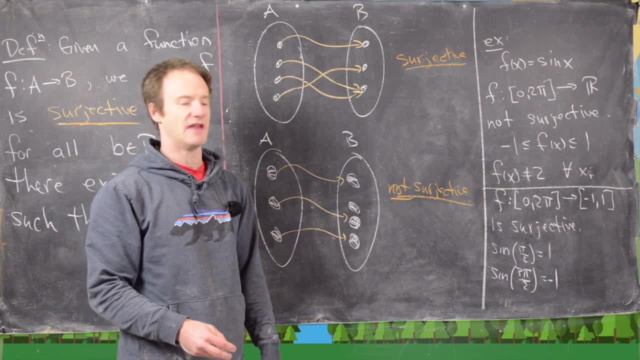 And so it achieves the largest number in the codomain and the smallest number in the codomain, But then, using the fact that sine is continuous and the intermediate value theorem will show that it maps on to every element of the codomain, Okay, good. 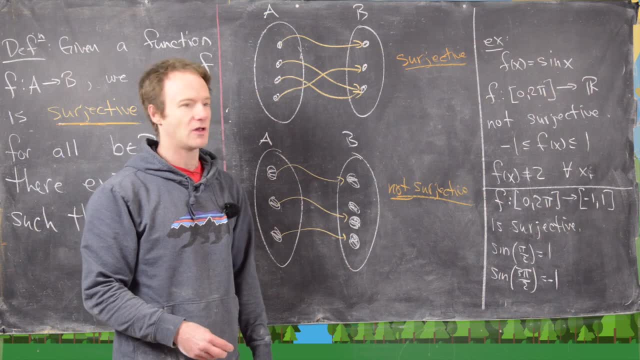 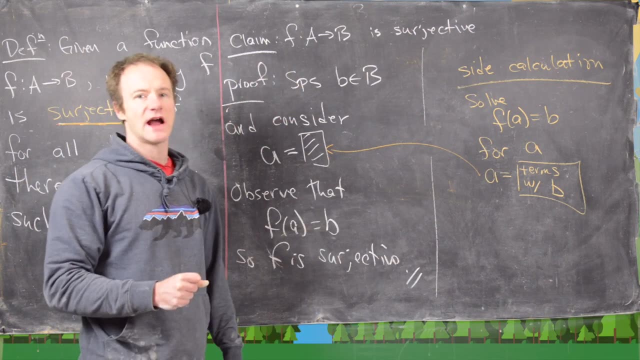 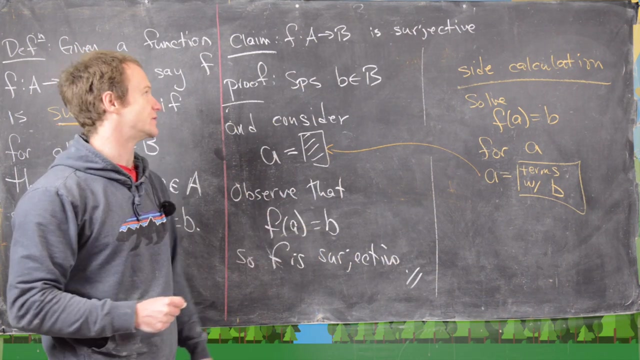 So I'm going to clean up the board and then we're going to look at an outline of a proof that a function is surjective. Okay, so let's look at the outline of a proof that some function is surjective. And it's really important that we look at this outline because there's a bit of a trick to it. 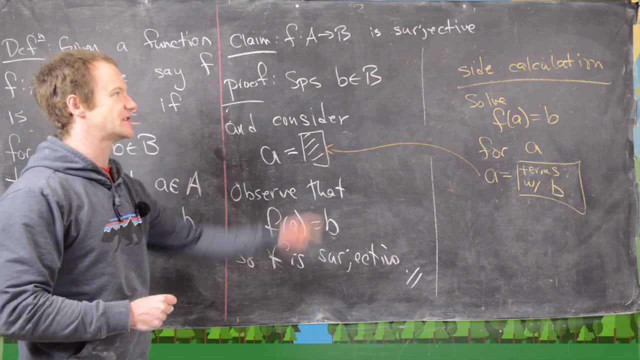 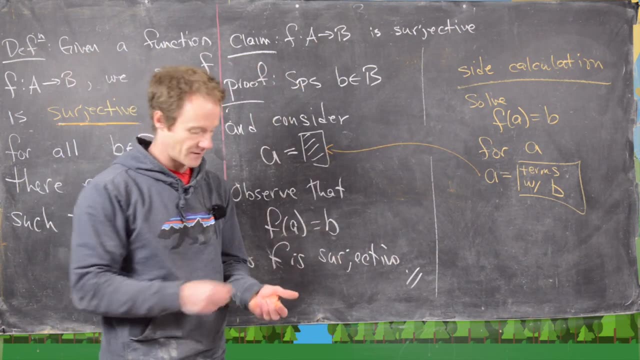 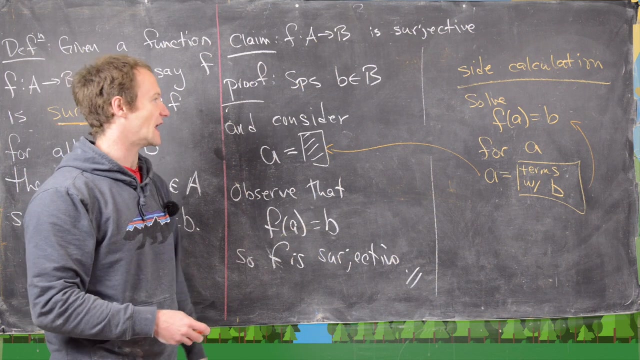 And so, Again, our claim is that f is surjective. And notice, there's this really important side calculation. So this side calculation is not in the proof And in fact, the side calculation in reverse will end up in the proof And it will end up in the proof at the end. 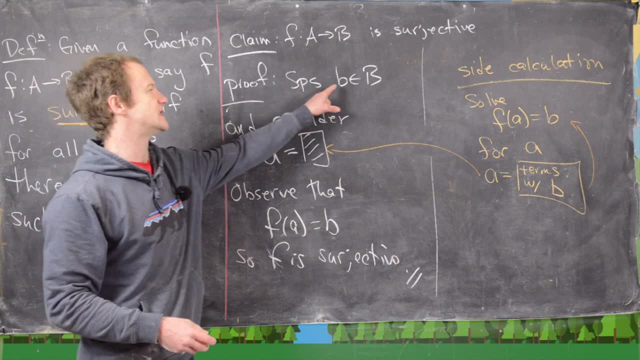 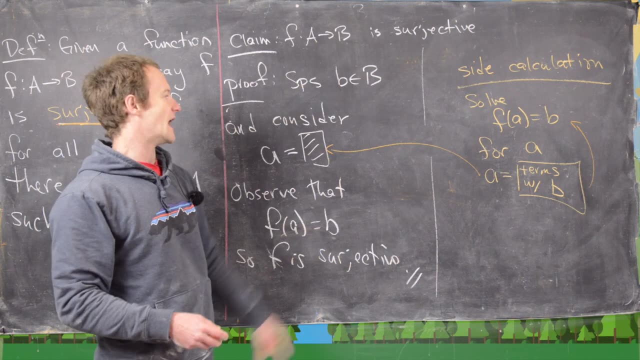 So let's look at the outline of the proof. So we suppose that b is in b And so b is an arbitrary element. And remember, our goal is to find an element a from the domain that's mapped. Okay, So we do that via this side calculation. 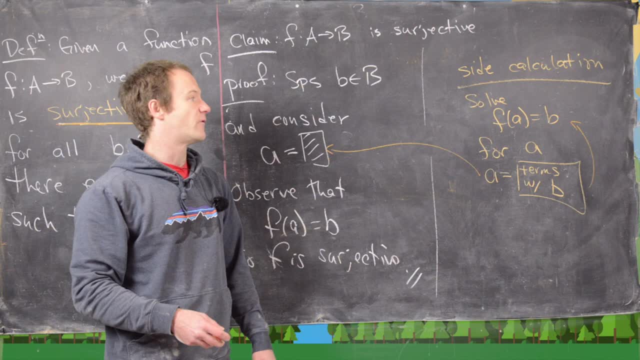 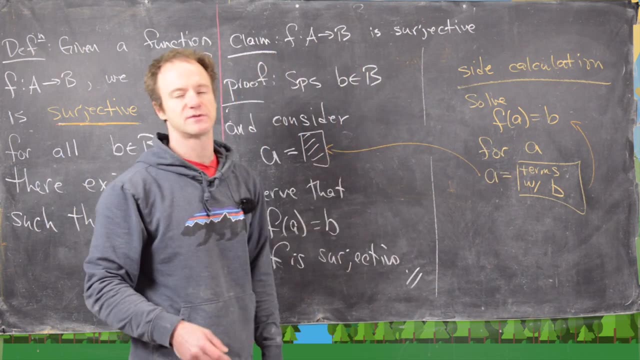 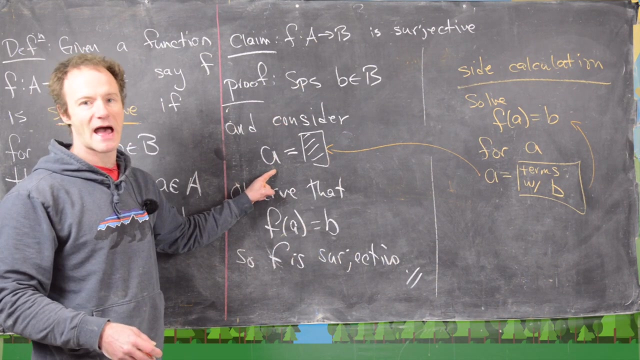 So we solve the equation f of a equals b for a, And so what that will give us is a equals some sort of combination of terms with b. Okay, great, Now we go back to the proof, And when we're writing up the proof, it seems like a little bit magical. 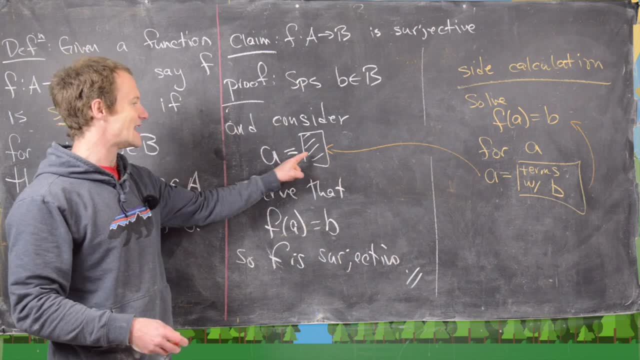 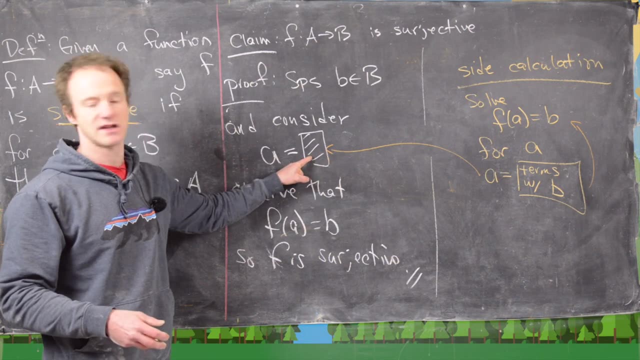 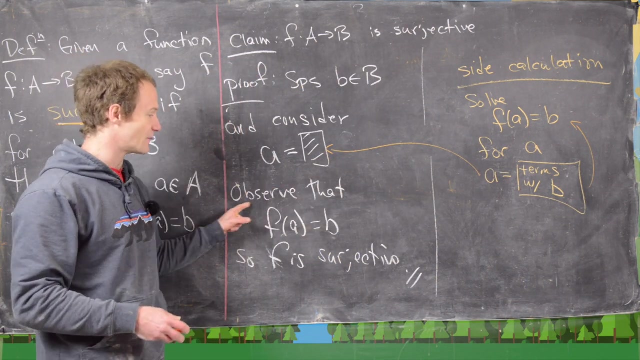 Because what we'll do is we'll consider a equal to just this complicated object Involving terms with this b, And so that's what we'll put here, What we got from our side- calculation, And the next thing that we want to do is say something like: observe that. 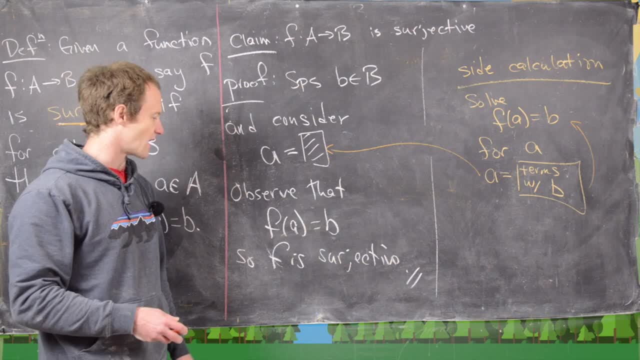 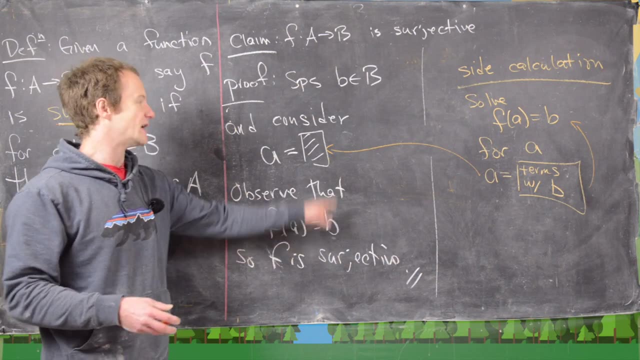 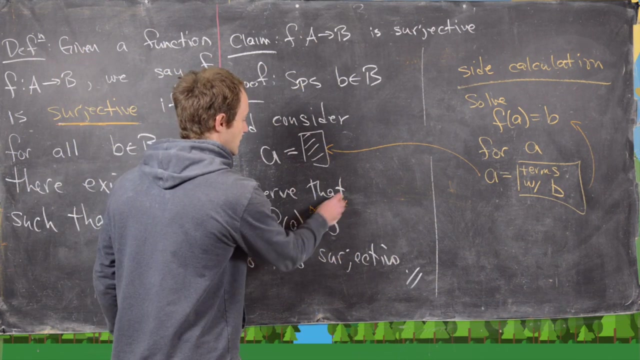 Or notice that Or something that relays that similar idea, That when you plug this value of a, which we've just grabbed from the ether, into our function, We get our arbitrary b from the codomain. And so- and in fact this calculation right here, 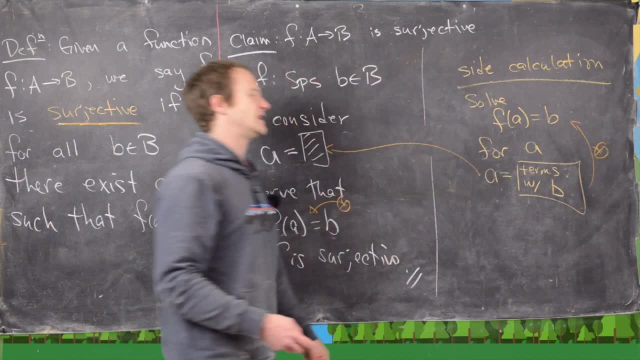 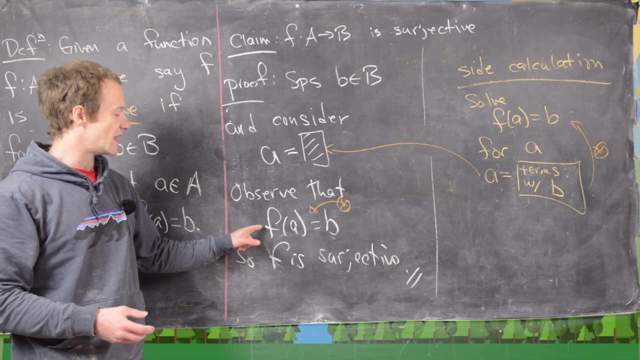 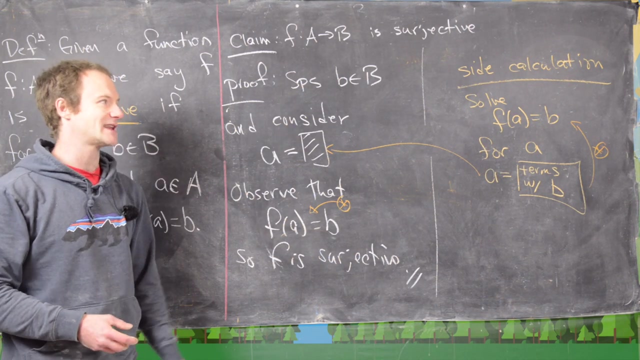 Is the reverse of what we did over here when we solved for a, And so that's how that side calculation shows up here. It shows up in reverse, But this equation right here shows that f is surjective. So again, it's really important to do this side calculation. 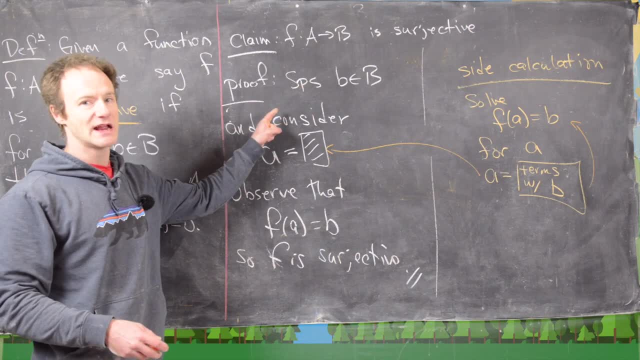 Okay, great. Now we go back to the proof. And when we're writing up the proof, it seems like a little bit magical. 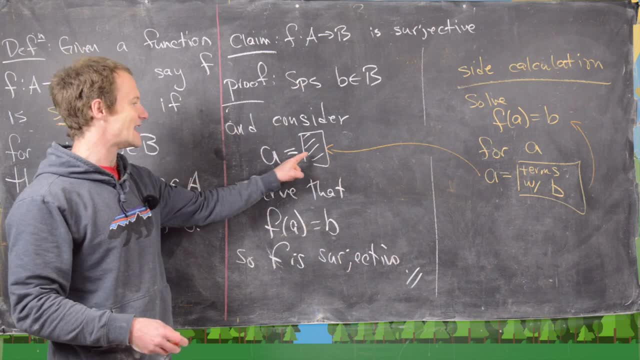 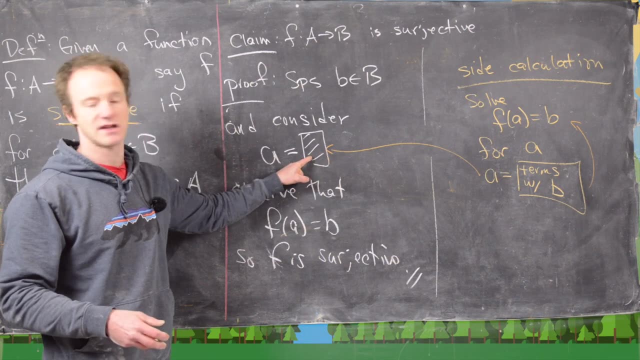 Because what we'll do is we'll consider a equal to just this complicated object. Involving terms with this b. 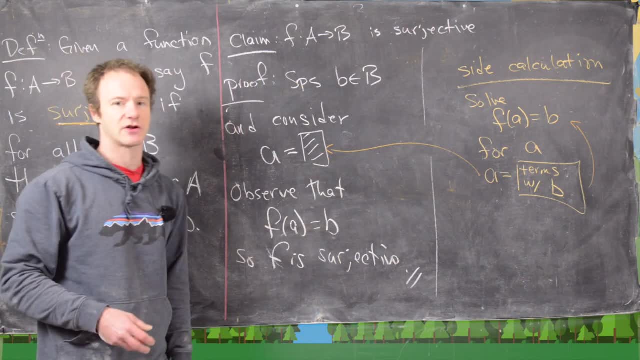 And so that's what we'll put here. What we got from our side calculation. 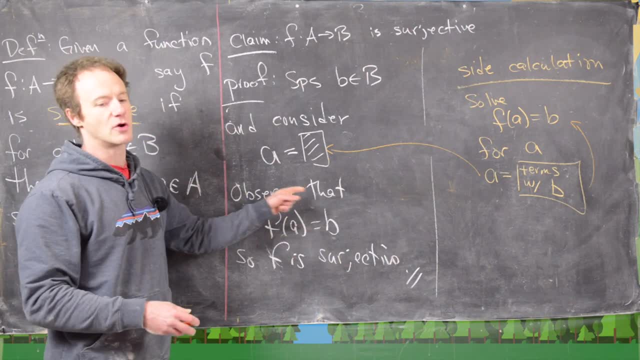 And the next thing that we want to do is say something like observe that. Or notice that. Or something that relays that similar idea. 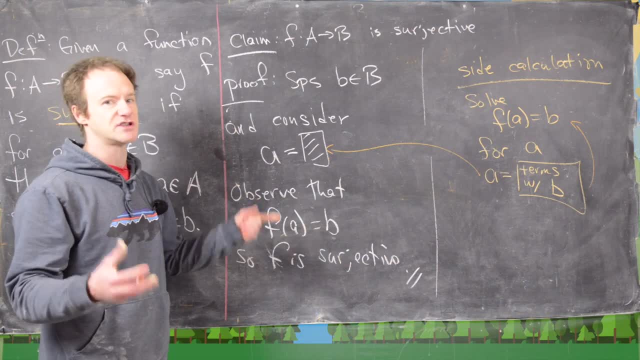 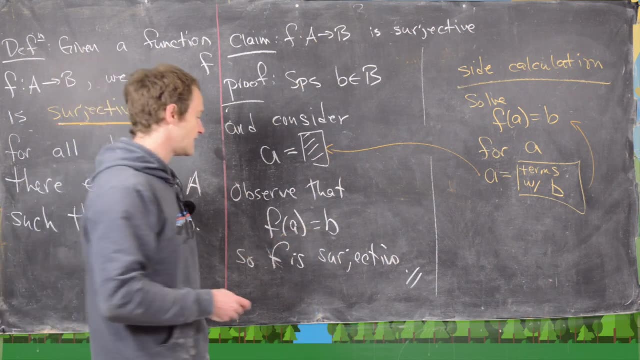 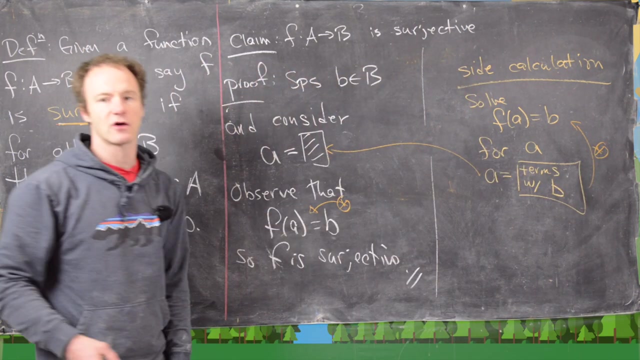 That when you plug this value of a, which we've just grabbed from the ether, into our function. We get our arbitrary b from the codomain. And so, and in fact, this calculation right here. Is the reverse of what we did over here when we solved for a. And so that's how that side calculation shows up here. It shows up in reverse. 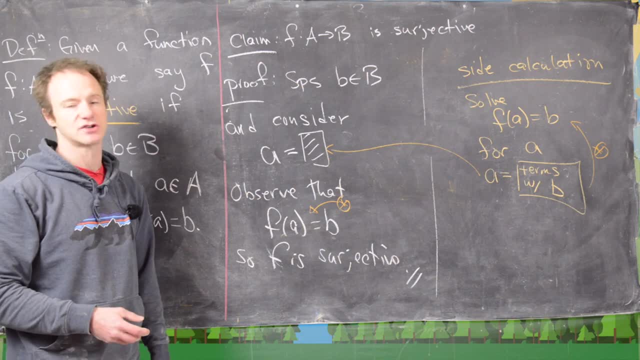 But this equation right here shows that f is surjective. So again, it's really important to do this side calculation. 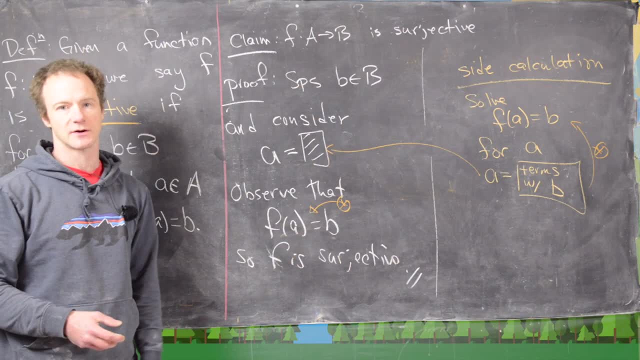 And not include it in the proof except in reverse down here. So when reading these types of proofs. 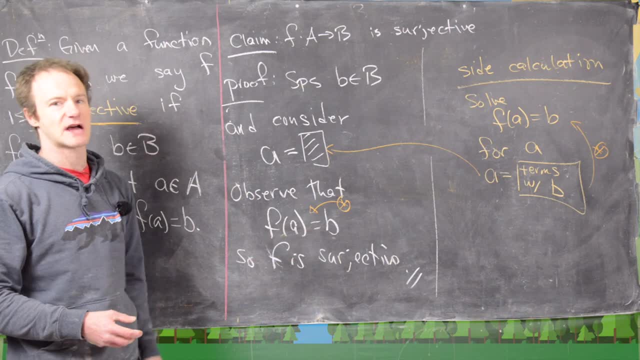 It should always be a little bit surprising when you're reading it from top to bottom. That this value of a is just kind of like given. Okay, good. 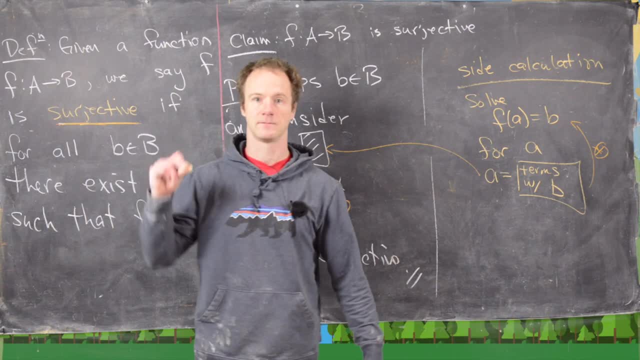 So now I'm going to clean up the board and we're going to look at some examples. Okay, so for our first example. 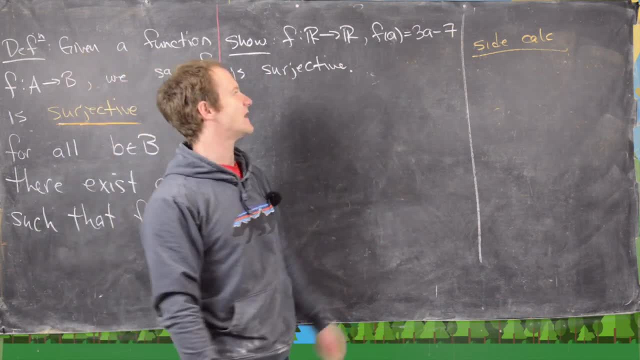 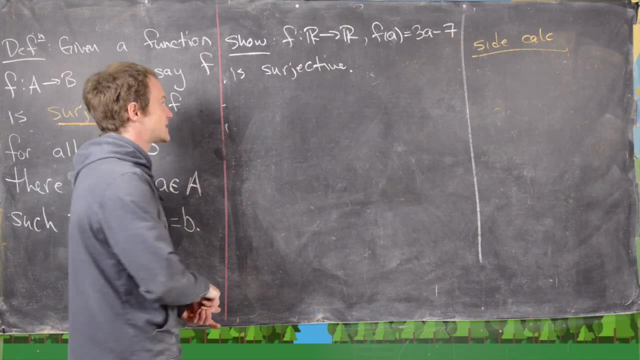 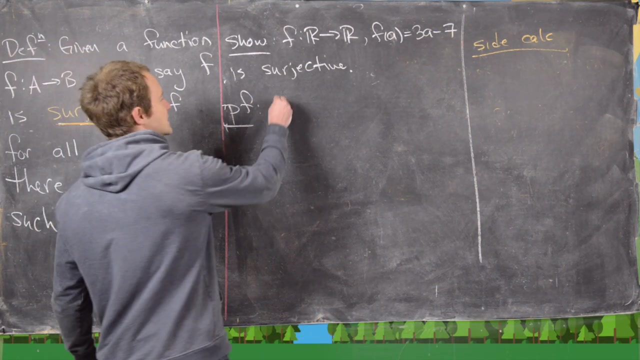 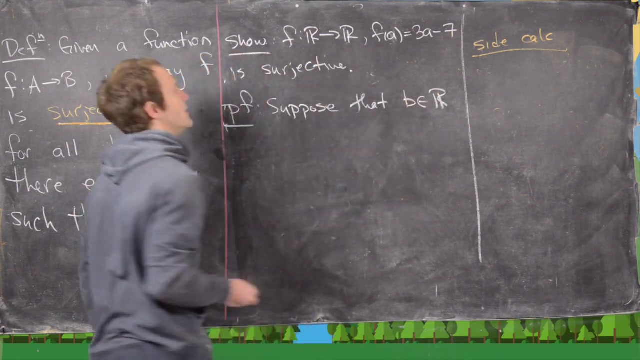 We'll consider the function from r to r given by f of a equals 3a minus 7. So in other words, that's just a line. We want to show that thing is surjective. So let's start our proof here. So our proof is going to start just the same way that we looked at in the outline. So let's suppose. That we have some element b from the codomain, which is r. 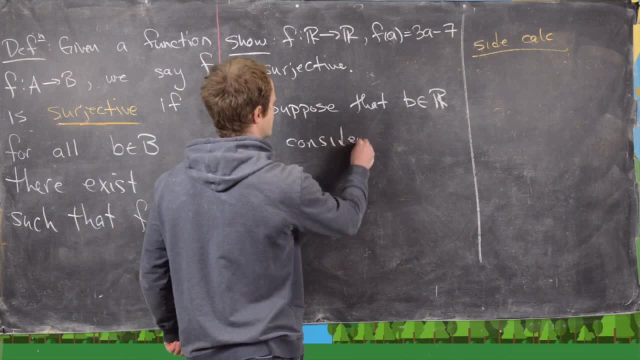 And we're going to consider a equals. 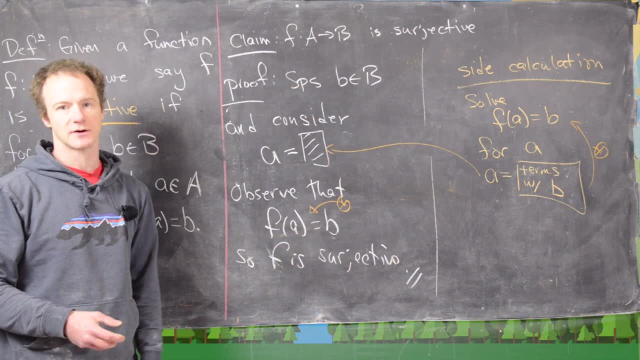 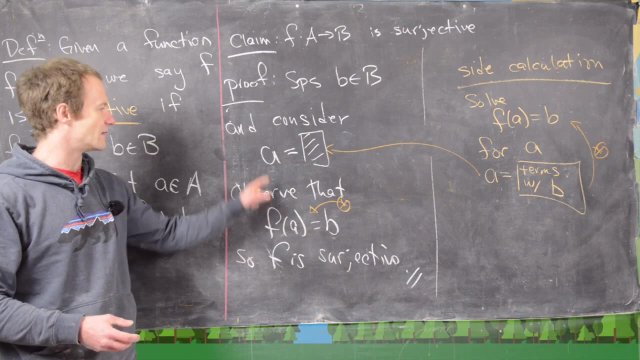 And not include it in the proof, except in reverse down here. So when reading these types of proofs, It should always be a little bit surprising- when you're reading it from top to bottom- That this value of a is just kind of like given. 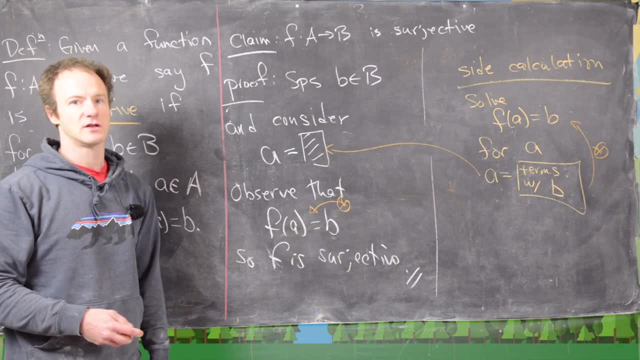 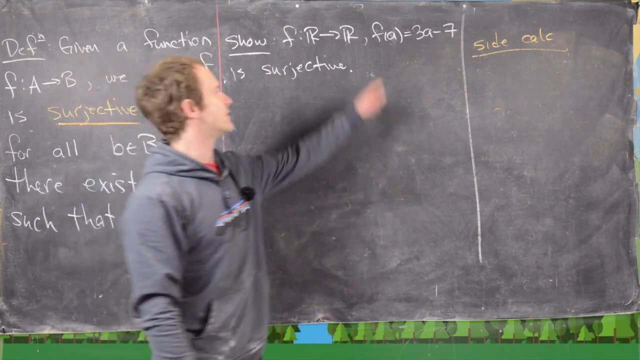 Okay, good. So now I'm going to clean up the board and we're going to look at some examples. Okay, so, for our first example, We'll consider the function from r to r, given by f, of a equals 3a minus 7.. 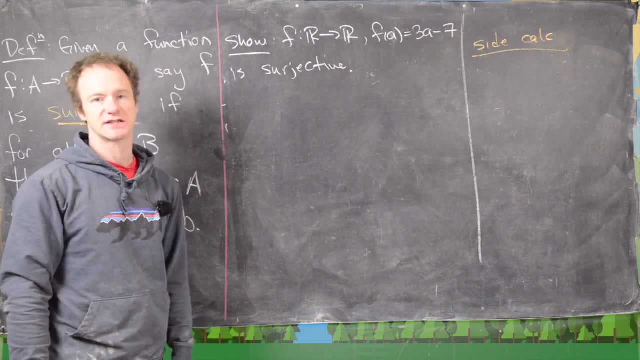 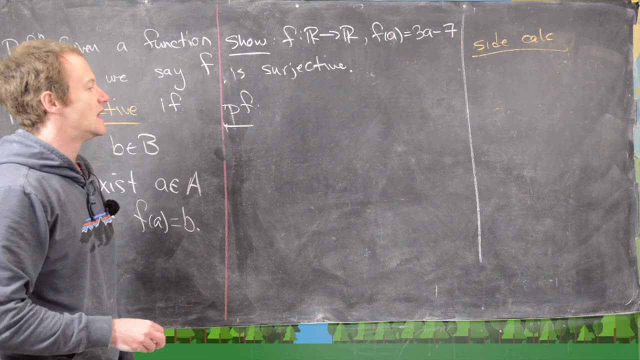 So, in other words, that's just a line We want to show. that thing is surjective. So let's start our proof here. So our proof is going to start just the same way that we looked at in the outline. So let's suppose 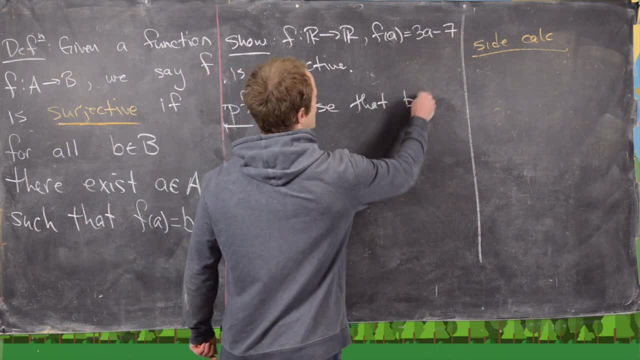 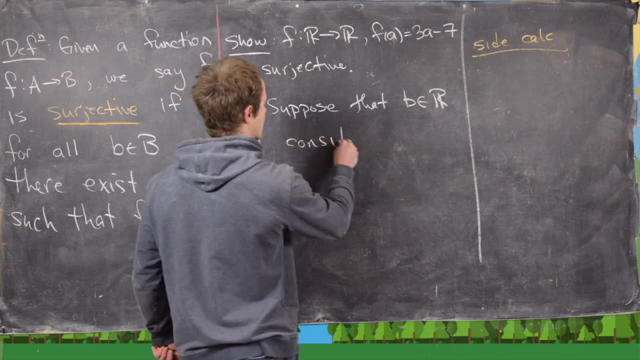 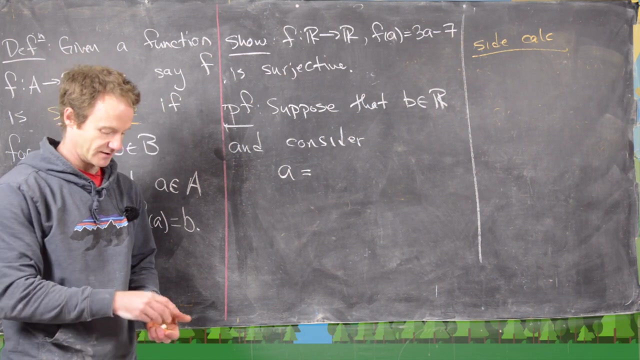 That we have some element b from the co-domain, which is r, And we're going to consider a equals. But now we have to stop because we need to input something from our side calculation Again. the side calculation won't show up in your solution that you hand in. 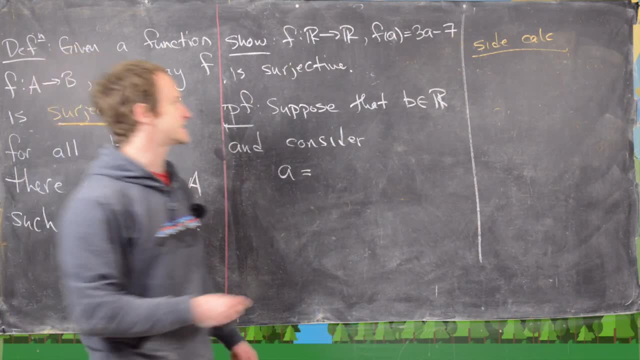 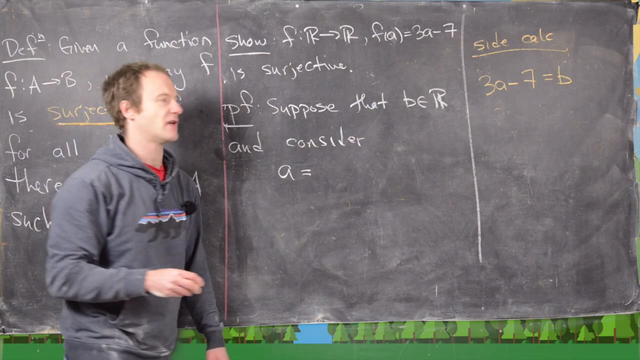 But it's important to do So. let's look at the side calculation. We want to solve 3a minus 7.. Minus 7 equals b, Recall. we want to solve: f of a equals b for a, And so you know that's not too hard to do in this case. 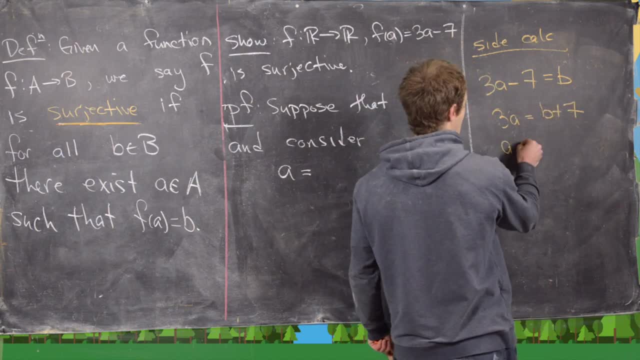 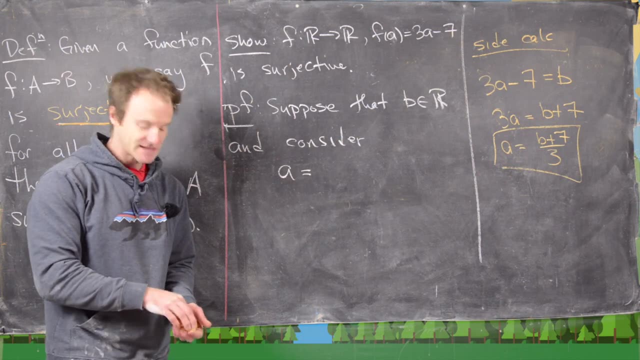 So we get 3a equals b plus 7.. Which makes a equal to b plus 7 over 3.. Great, So that's the value of a that we're going to consider right here. So we'll say b plus 7 over a. 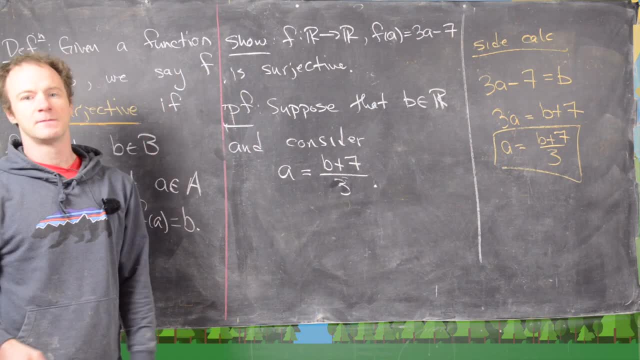 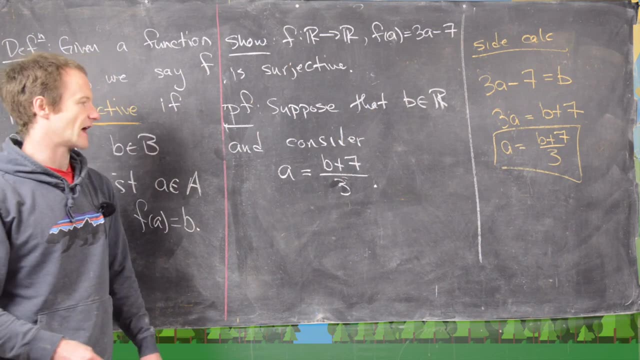 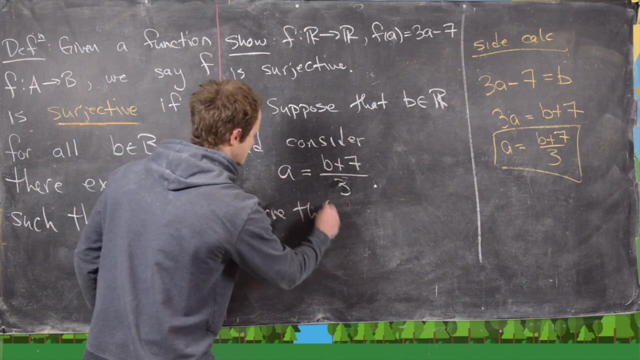 Sorry, over 3.. Good, And notice, that's going to be a real number for any b, just by kind of its obvious fact. And so now the next thing that we'll do is we'll observe that if we do f of a. 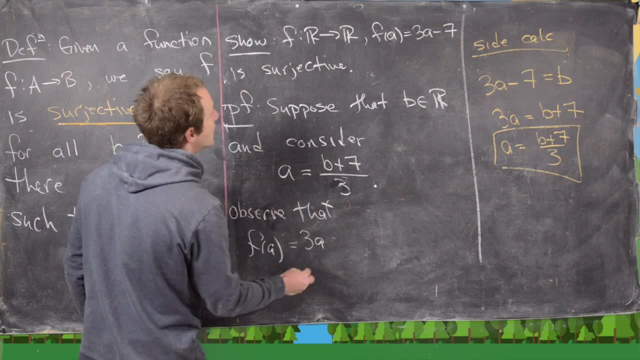 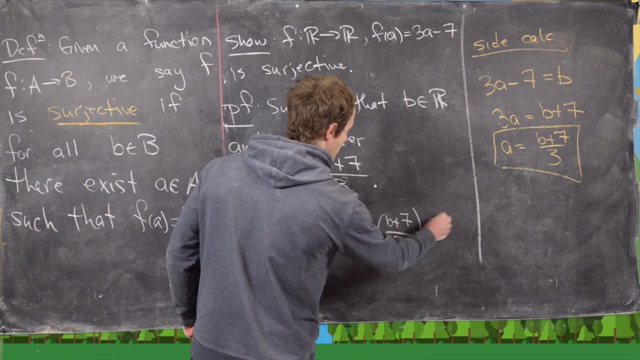 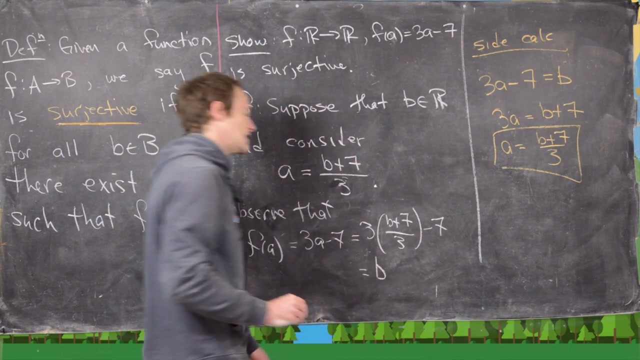 That's going to be 3a minus 7.. But that's going to be equal to 3 times b plus 7 over 3 minus 7.. By the value of a, By the value of a that we constructed, But that's going to be exactly b by simple algebra. 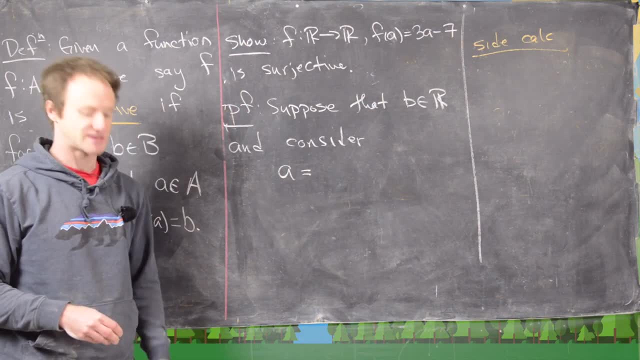 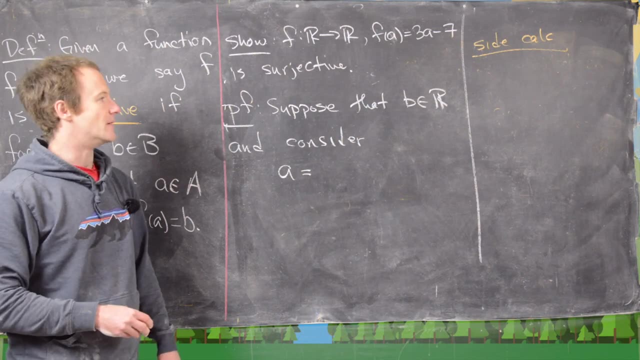 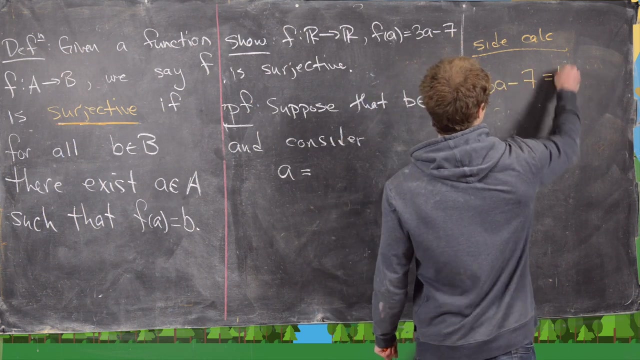 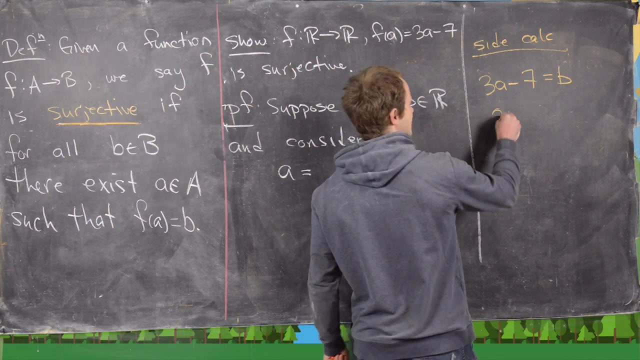 But now we have to stop because we need to input something from our side calculation. Again, the side calculation won't show up in your solution that you hand in. But it's important to do. So let's look at the side calculation. We want to solve 3a. Minus 7 equals b. Recall we want to solve f of a equals b for a. And so, you know, that's not too hard to do in this case. 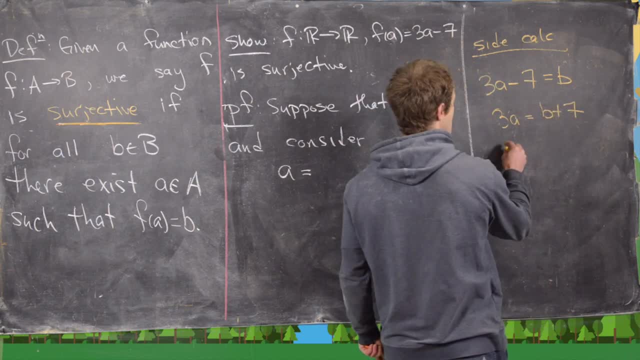 So we get 3a equals b plus 7, which makes a equal to b plus 7 over 3. Great. 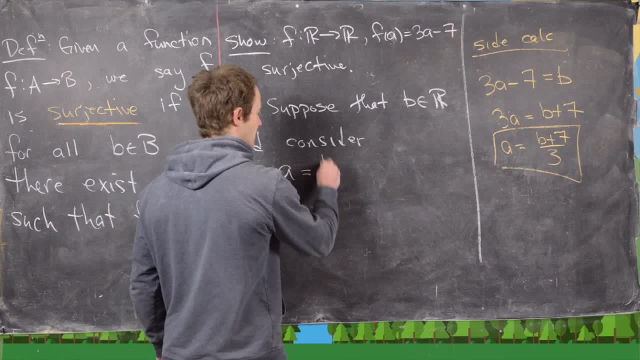 So that's the value of a that we're going to consider right here. 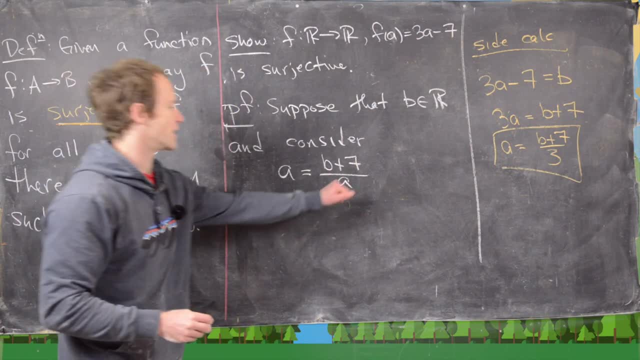 So we'll say b plus 7 over a. Sorry, over 3. Good. 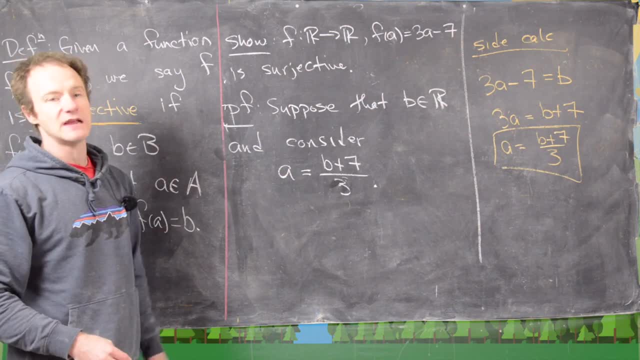 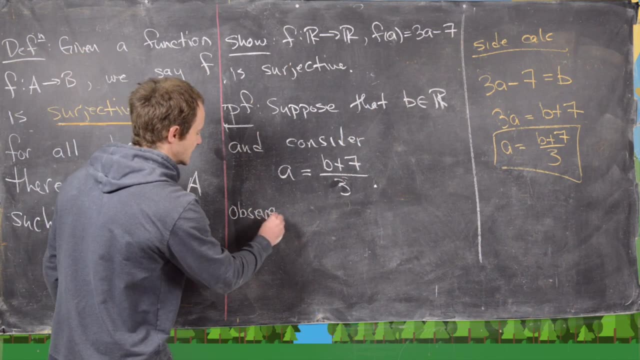 And notice that's going to be a real number for any b just by kind of its obvious fact. And so now the next thing that we'll do is we'll observe that if we do f of a, 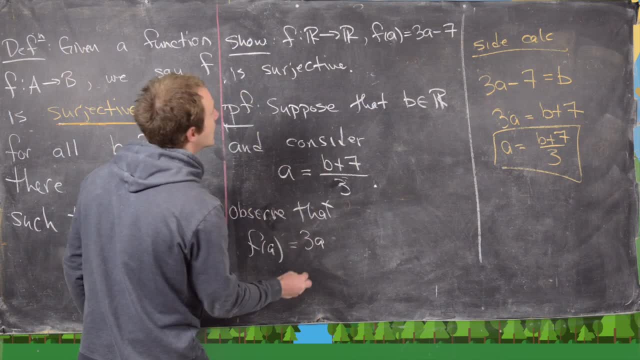 that's going to be 3a minus 7. 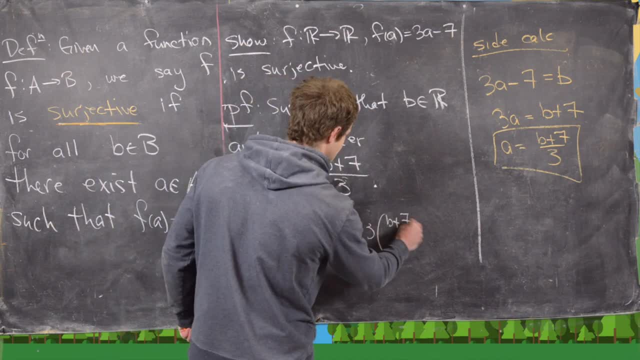 But that's going to be equal to 3 times b plus 7 over 3 minus 7. Okay. So that's going to be 3a minus 7. So that's going to be the value of a that we constructed. 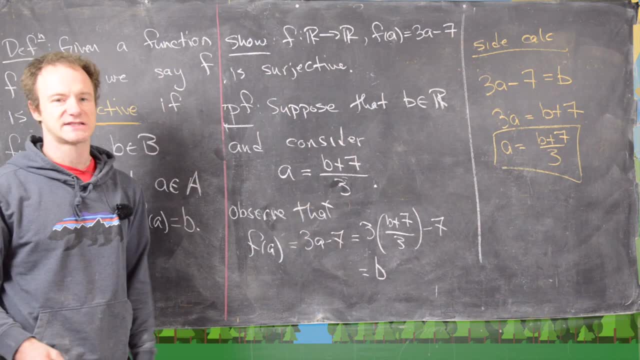 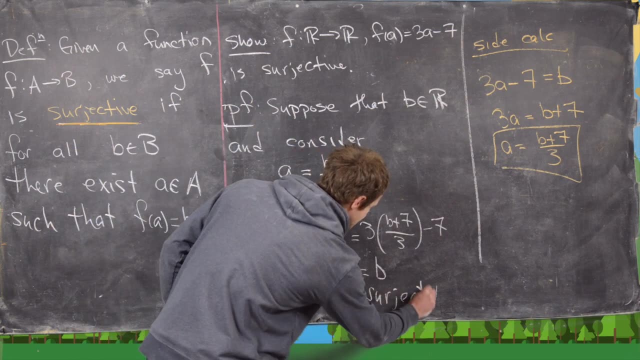 But that's going to be exactly b by simple algebra. But that means that f is surjective. 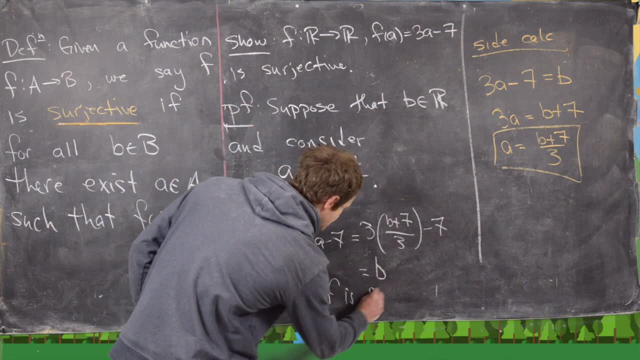 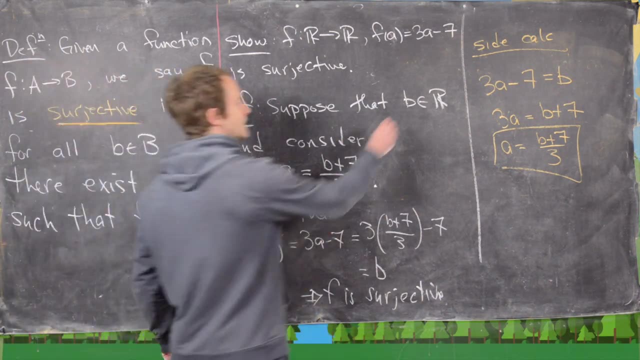 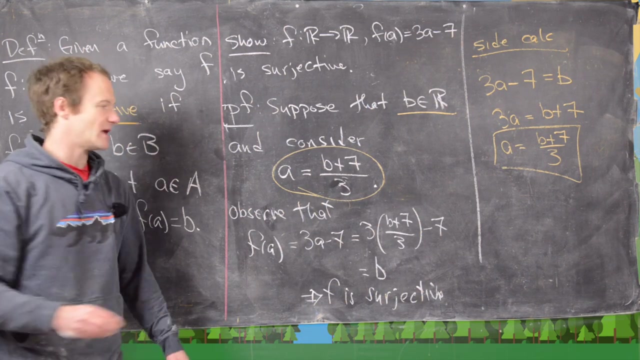 But that means that f is surjective. And let's see Why does it mean that f is surjective? Because what we've done is we've taken an arbitrary element from the codomain, We've constructed an element from the domain And we stick that element from the domain into the function. 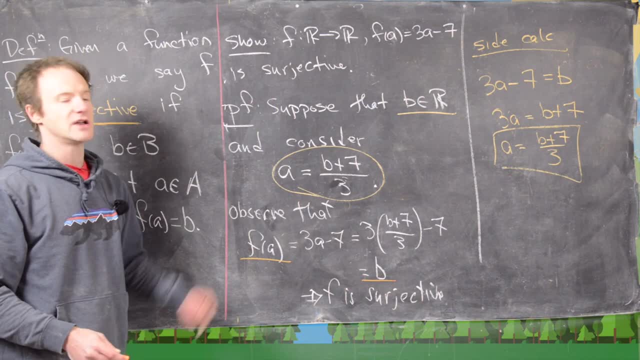 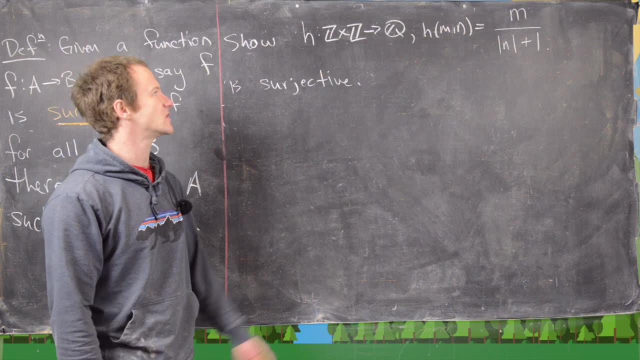 We get our arbitrary element from the codomain. Okay, good, I'm going to clean up the board and then we're going to do one more example, Okay, So for our final example, we'll look at the following function: So we've got h, which goes from z cross z to q. 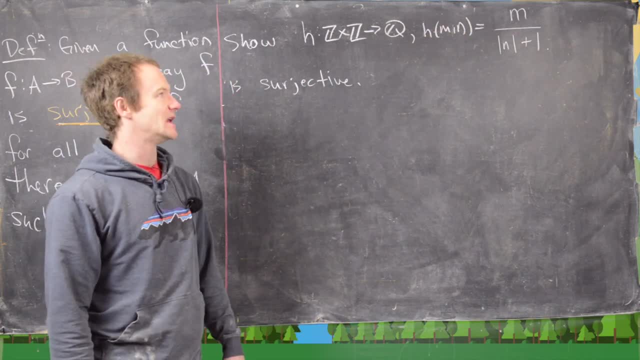 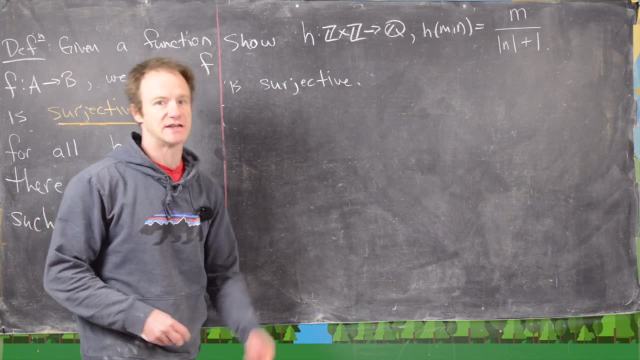 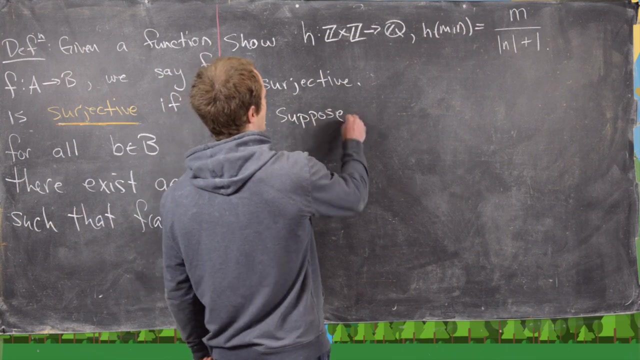 And it's defined by h of mn equals m over the absolute value of n plus 1.. We want to show that this function is surjective, So we'll use the same outline that we've been using. So let's suppose that we have some element from the codomain. 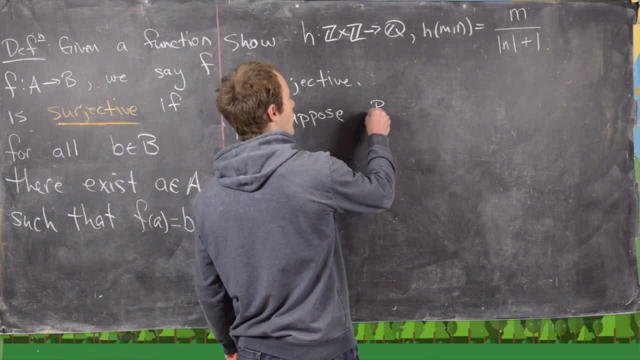 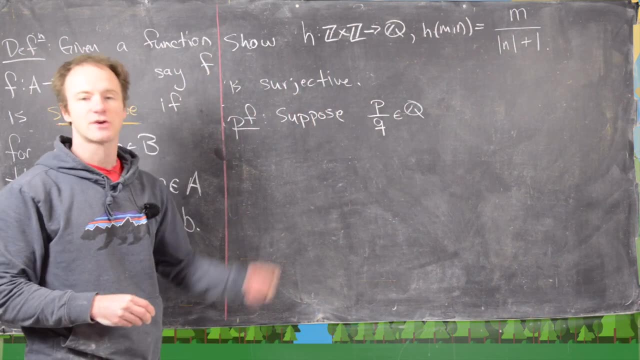 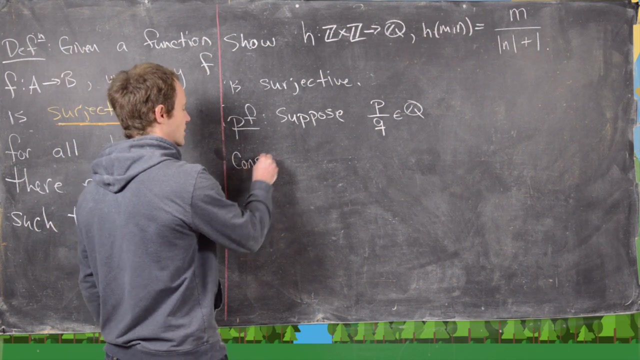 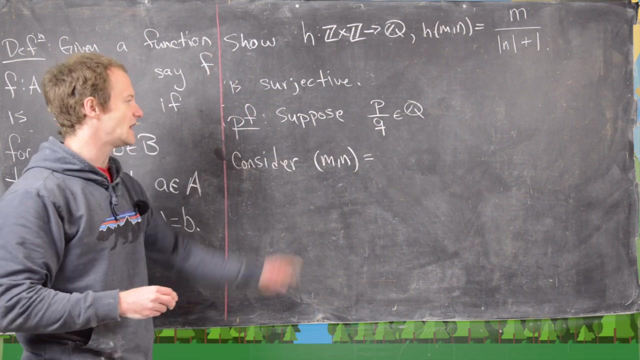 In other words from q, So we can always write elements of the rational numbers as p over q. Great, And so here we're, using the structure of the rational numbers, And the next thing that we want to do is consider m- n equals, but now we don't know what this needs to be equal to. 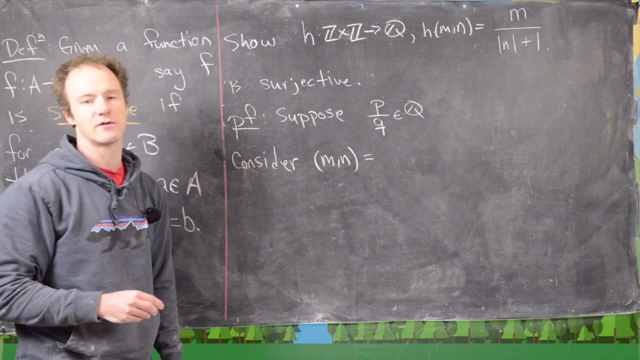 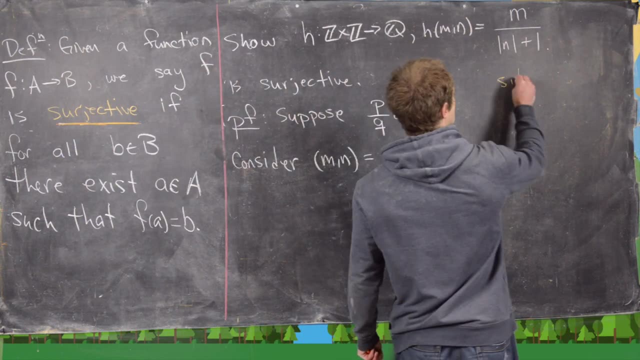 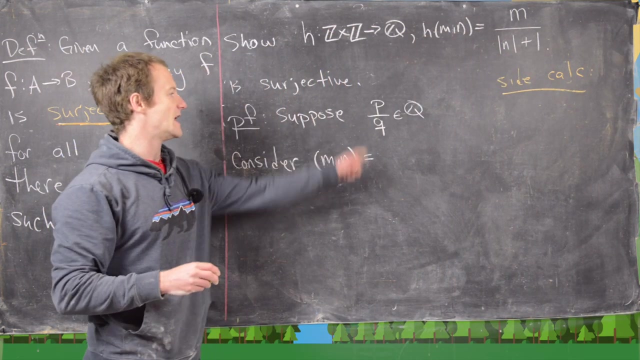 We do know that when we plug this into the function, we should get p over q. So now what we'll do is do our side calculation, Which is setting h of m comma n equal to p over q. In other words, we want to set m over absolute value n plus 1. 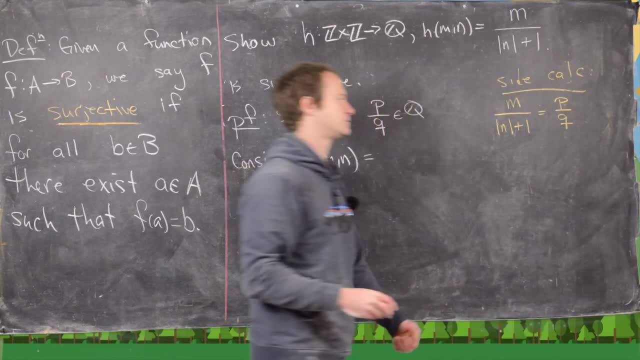 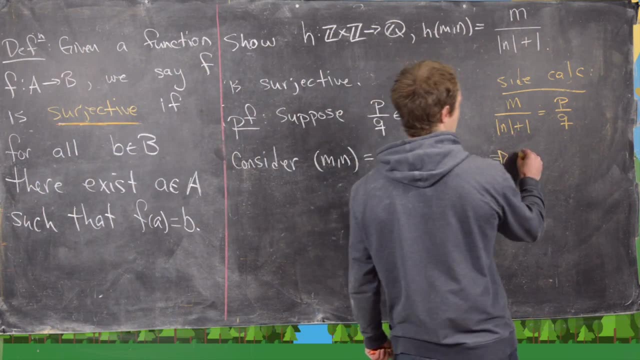 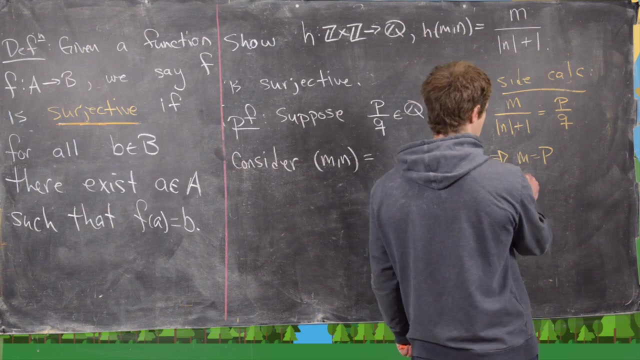 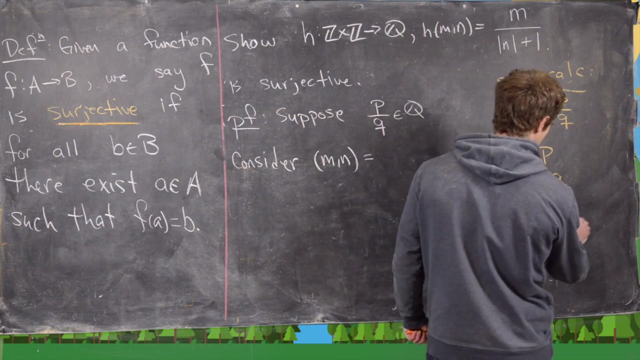 equals p over q, Okay, good. But now notice this is going to be equal. if m equals p, Great. And then notice that the absolute value of n plus 1 can be equal to q, Which means that the absolute value of n equals q minus 1.. And let's see. 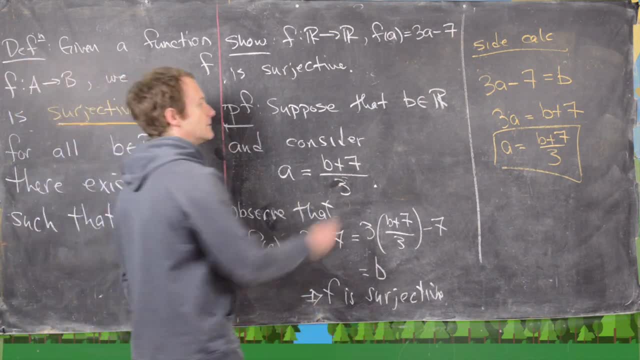 Why does it mean that f is surjective? Because what we've done is we've taken an arbitrary element from the codomain. 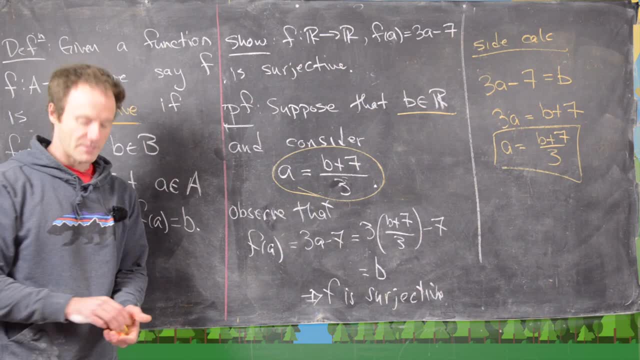 We've constructed an element from the domain that when we stick that element from the domain into the function, we get a value of a. And then we get our arbitrary element from the codomain. Okay, good. I'm going to clean up the board, and then we're going to do one more example. Okay. 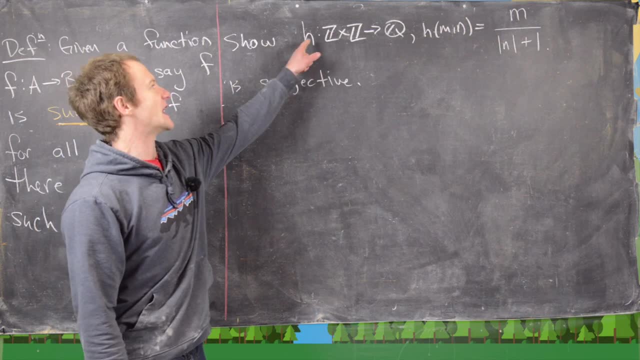 So for our final example, we'll look at the following function. So we've got h, which goes from z cross z to q. 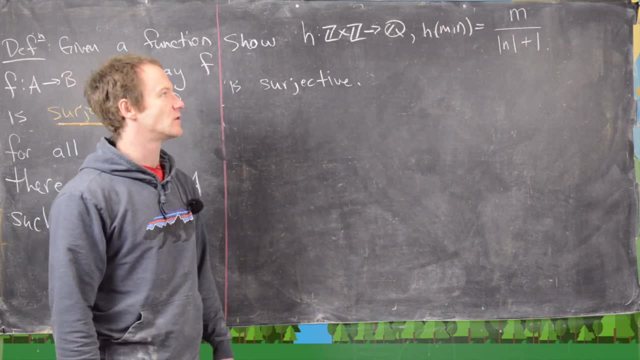 And it's defined by h of mn equals m over the absolute value of n plus 1. 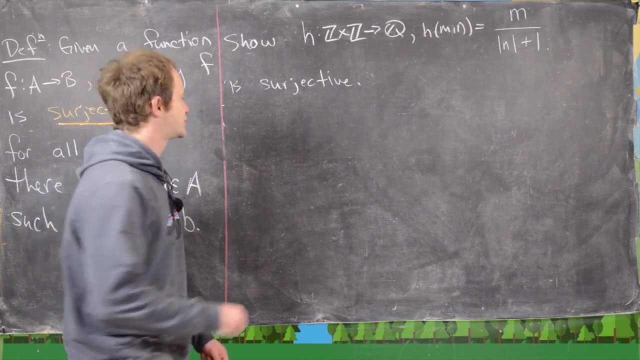 We want to show that this function is surjective. So we'll use the same outline that we've been using. 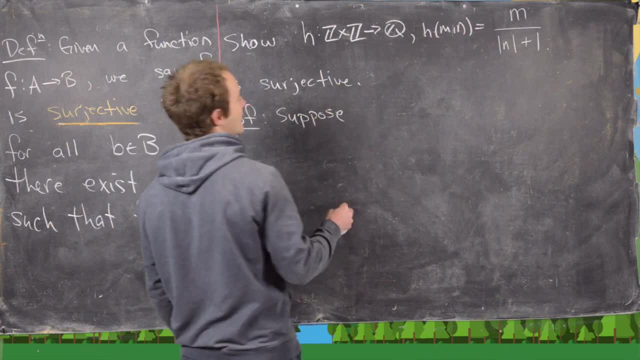 So let's... Let's suppose that we have some element from the codomain, in other words, from q. 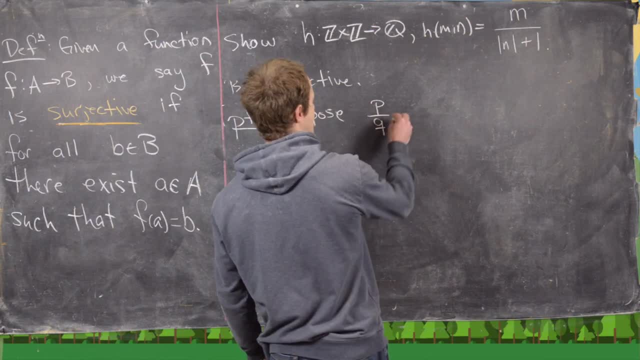 So we can always write elements of the rational numbers as p over q. Great. 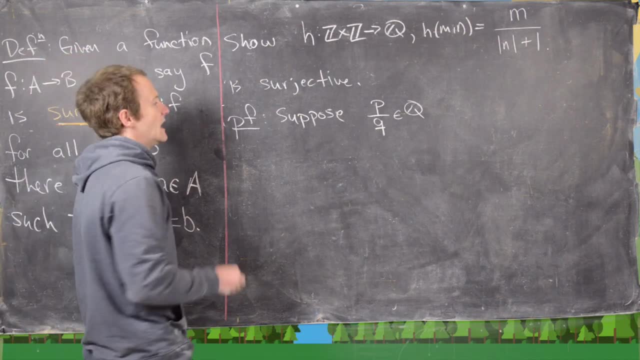 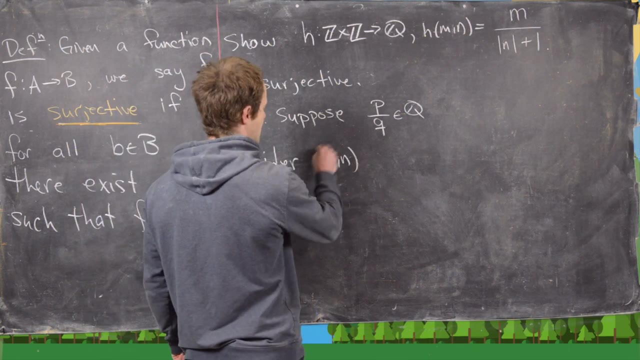 And so here we're using the structure of the rational numbers. And the next thing that we want to do is consider m comma n equals... But now we don't know what this means. It needs to be equal to. 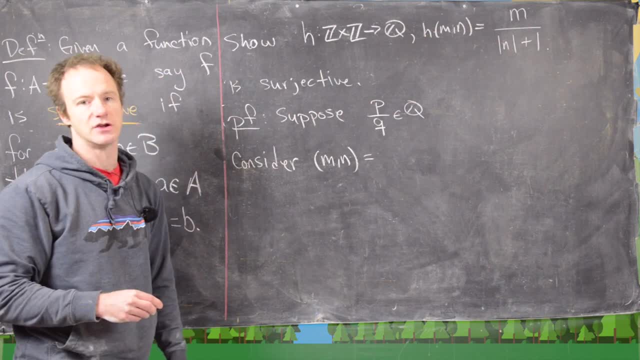 We do know that when we plug this into the function, we should get p over q. So now what we'll do is do our side calculation. 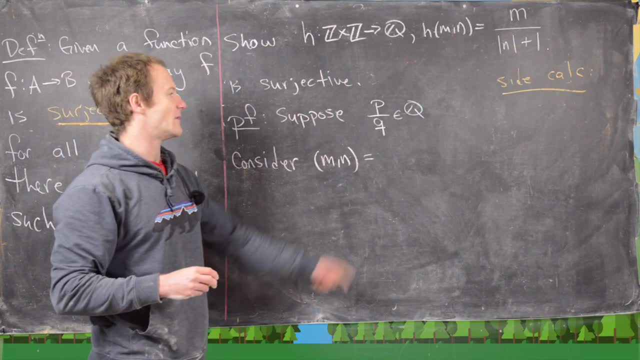 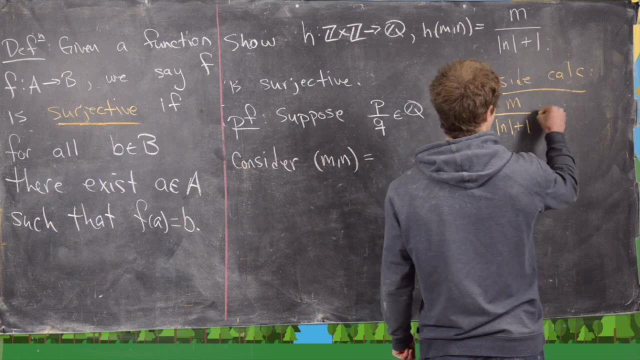 Which is setting h of m comma n equal to p over q. In other words, we want to set m over absolute value n plus 1 equal to p over q. Okay. Good. 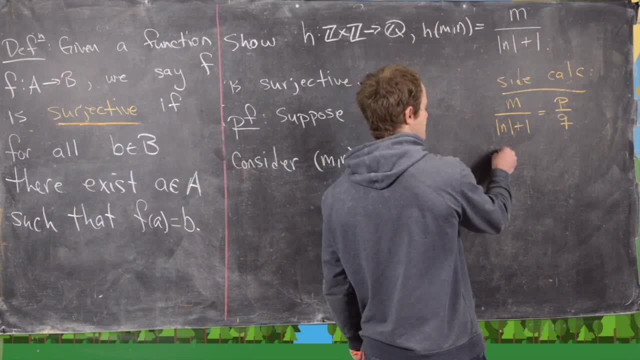 But now notice this is going to be equal if m equals p. Great. 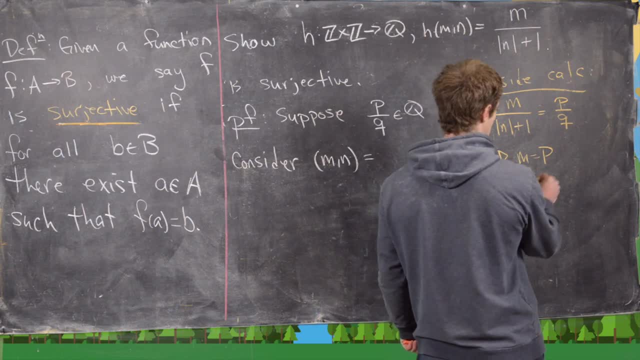 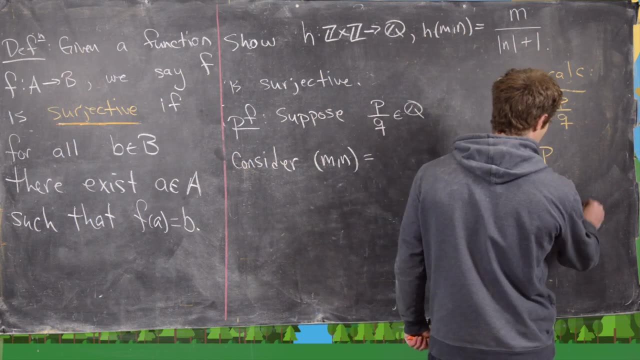 And then notice that the absolute value of n plus 1 can be equal to q, which means that the absolute value of n equals q minus 1. Good. 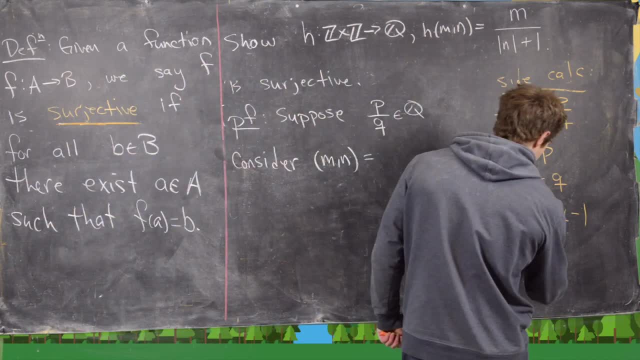 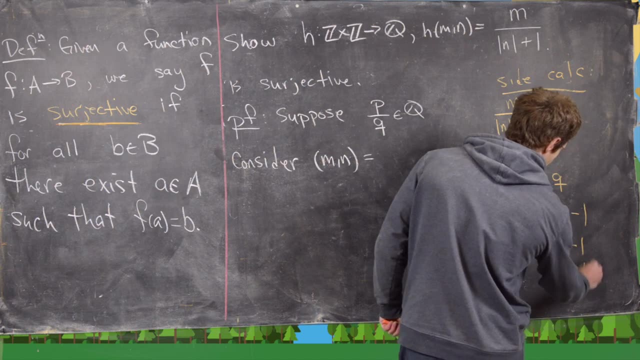 In other words, we have n equals either... q minus 1 or negative q minus 1. That's what it means for the absolute value of n to equal q minus 1. 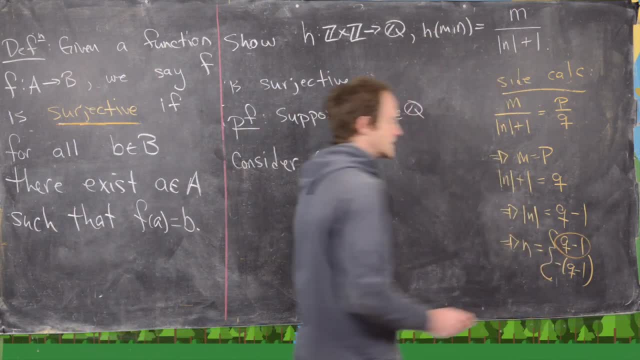 But we might as well take this first one because we want one element that's going to be mapped to p over q, not all elements. That's all we need to show this thing is surjective. 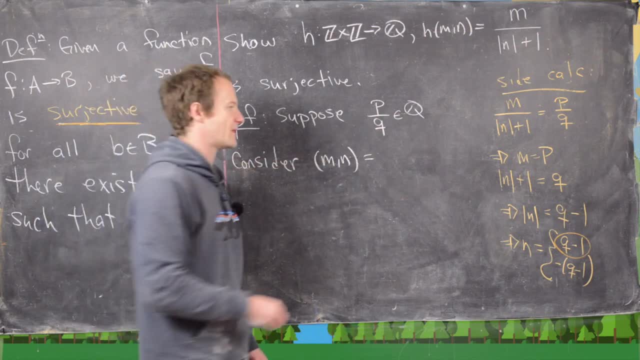 So again, we'll set m comma n equal to what we got from that over there. So this is going to be p and then q minus 1. Okay. 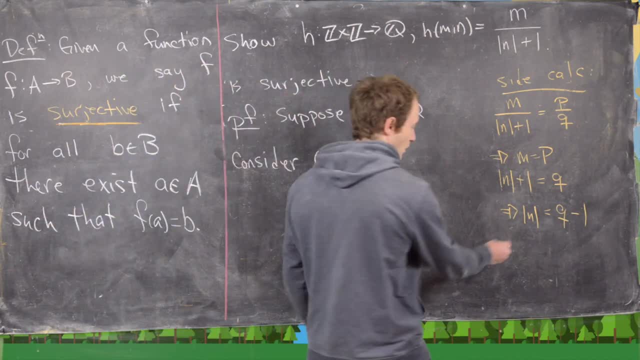 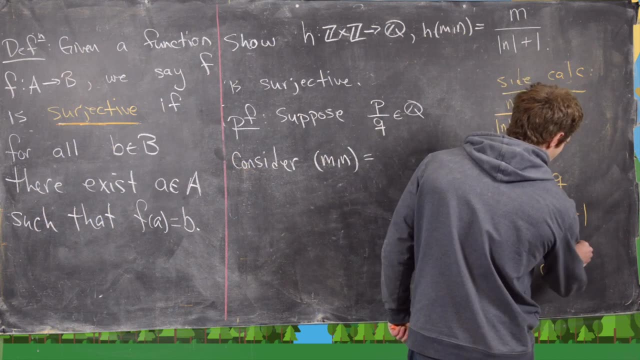 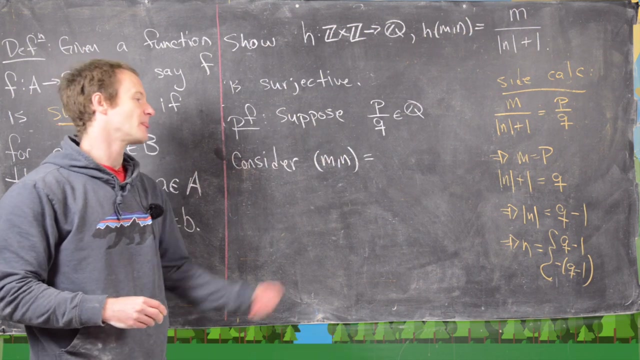 Good. In other words, we have n equals either q minus 1 or negative q minus 1.. That's what it means for the absolute value of n to equal q minus 1.. But we might as well take this first one. 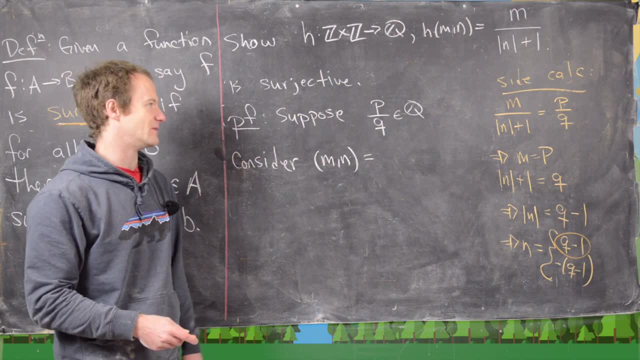 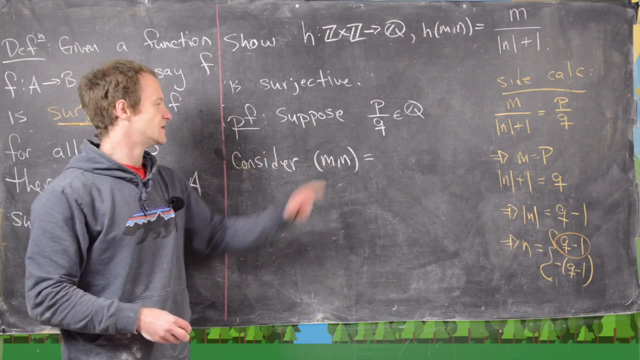 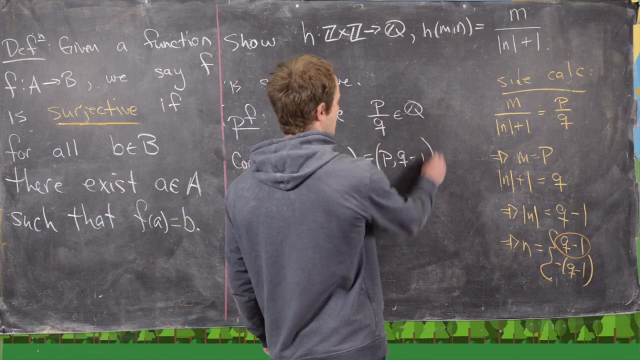 because we want one element that's going to be mapped to p over q, not all elements. That's all we need to show. this thing is surjective. So again, we'll set m comma n, equal to what we got from this. So this is going to be p and then q minus 1.. 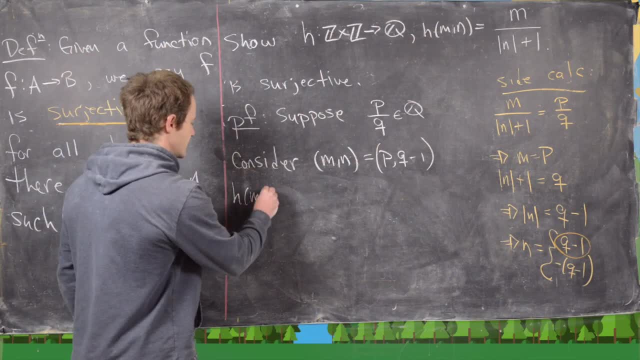 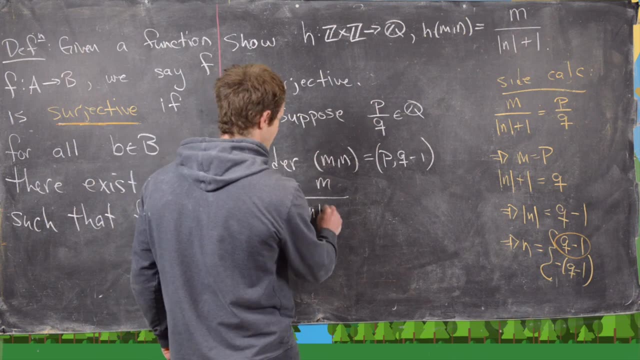 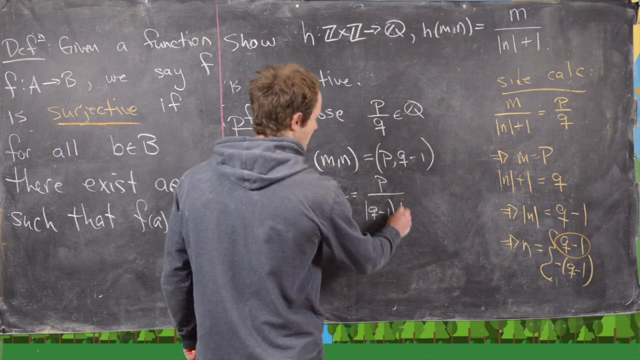 Okay, so now we'll finish it off. So let's plug this value into h, So we have h of m- n. So that's going to be equal to m over absolute value of n plus 1.. So that's going to be equal to p over absolute value of q minus 1 plus 1.. 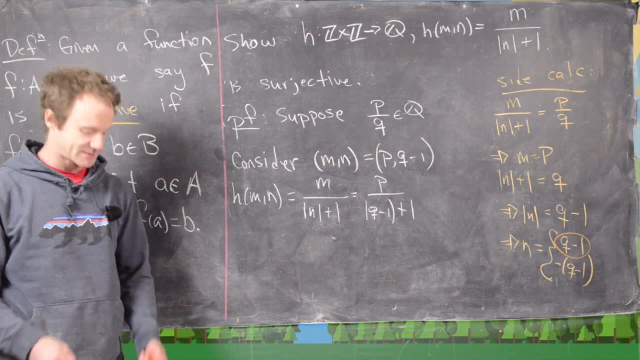 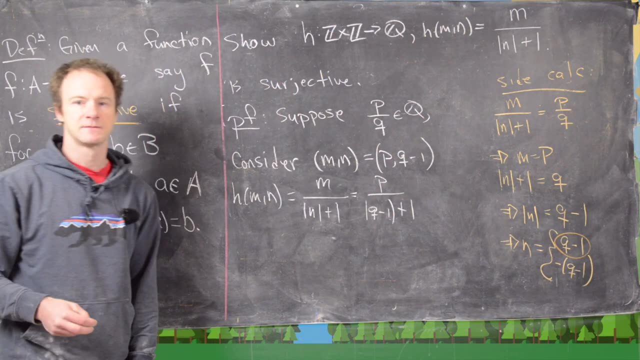 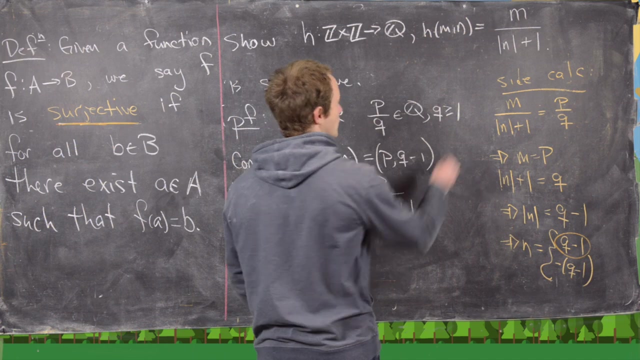 Okay, So now we might be a little stuck with these absolute values, But notice what we can do up here in order to unstick ourselves, And that is, we could have started from the beginning assuming that q is bigger than or equal to 1.. 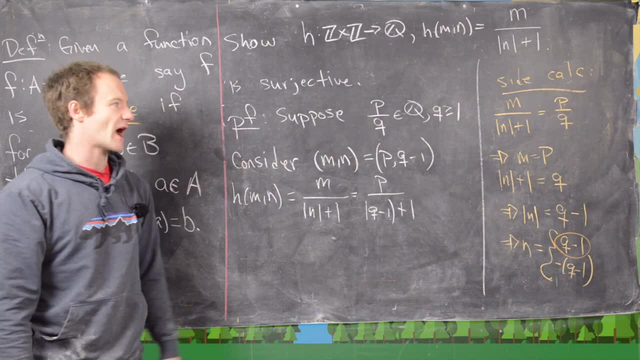 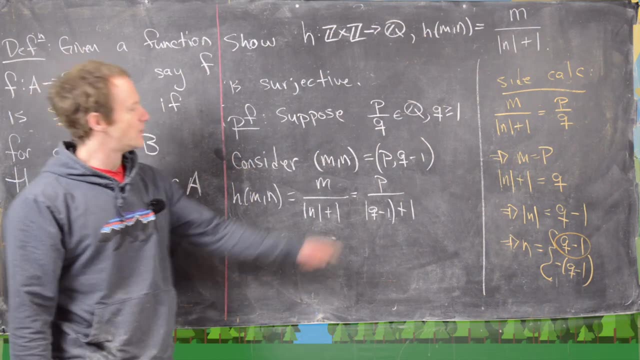 Right. So we know that when we write a rational number as a ratio of integers, this q has to be not equal to 0. But it could be positive or negative. But if it's negative we could just take that negative and absorb it into the p upstairs. 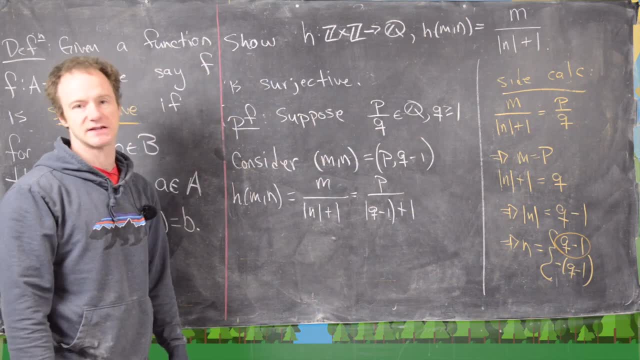 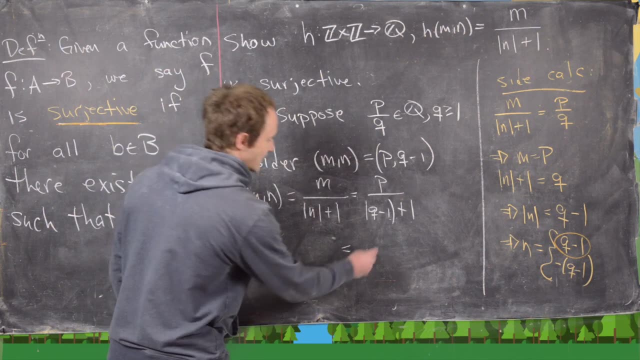 meaning that we can always assume that q is positive. Great. But if q is positive, then q minus 1 is non-negative, which means we can get rid of those absolute value signs, which means we get this as q minus 1, plus 1 or p over q. 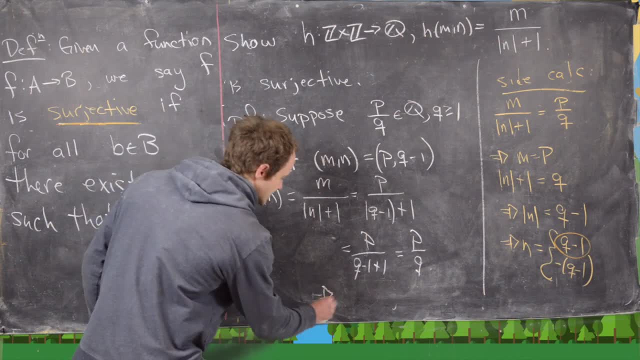 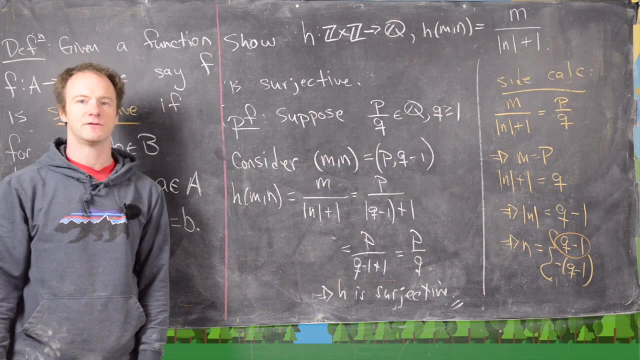 Great, But that's exactly what we need: to show that h is surjective, and that finishes our proof. Okay, that's a good place to end this video. 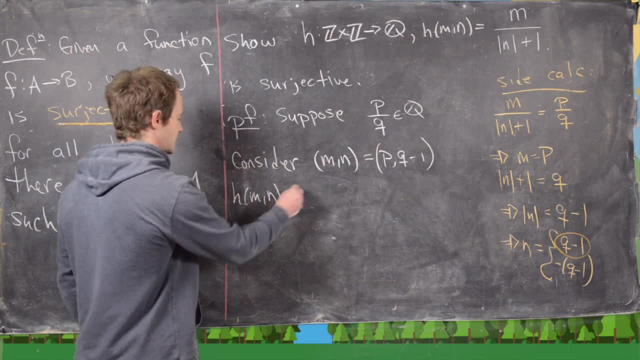 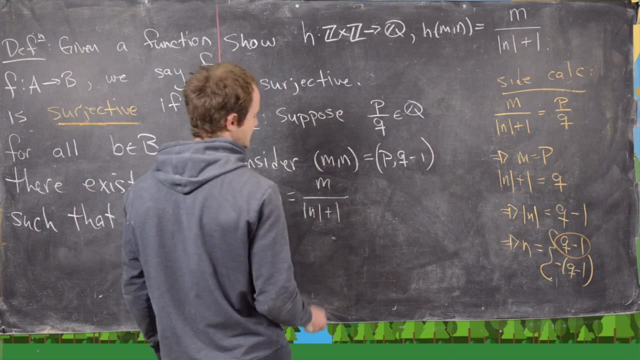 So now we'll finish it off. So let's plug this value into h. So we have h of m n. So that's going to be equal to m over absolute value of n plus 1. 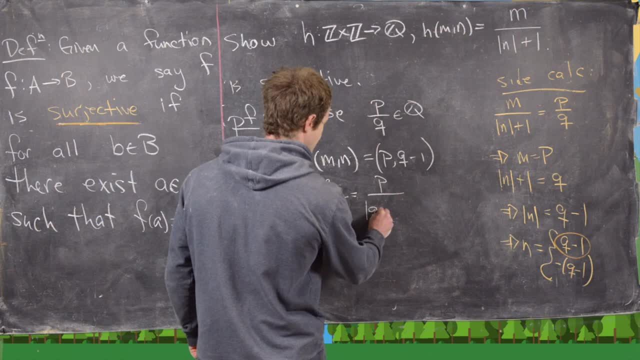 So that's going to be equal to p over absolute value of q minus 1 plus 1. Okay. 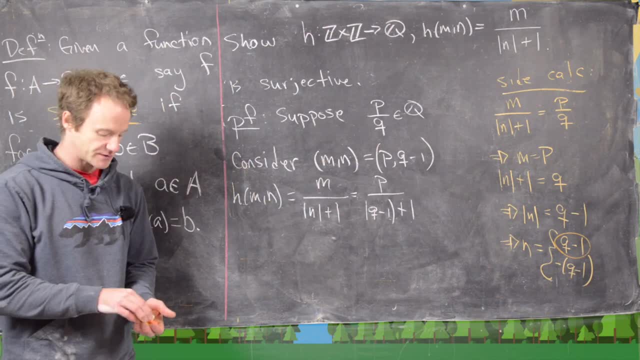 So now we might be a little stuck with these absolute values. 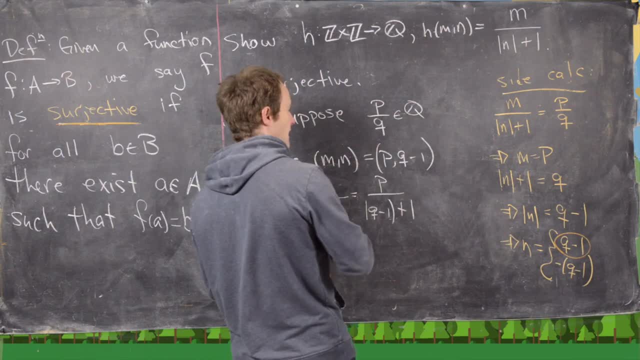 But notice what we can do up here in order to unstick ourselves. 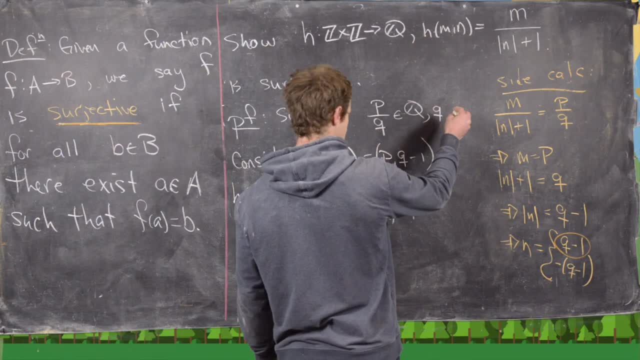 And that is we could have started from the beginning assuming that q is bigger than or equal to 1. Right? 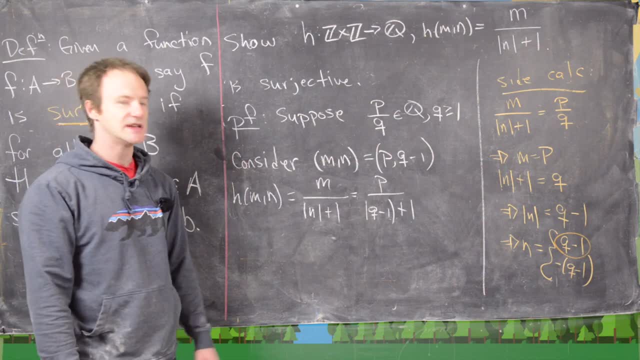 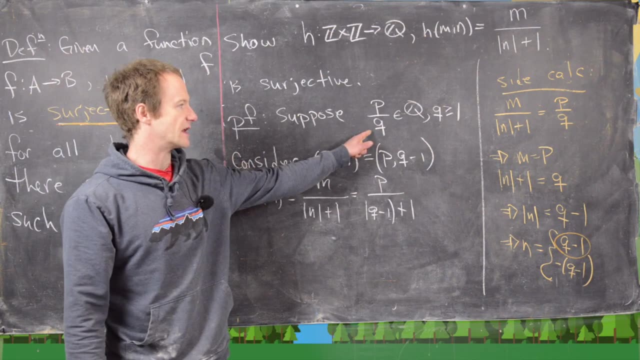 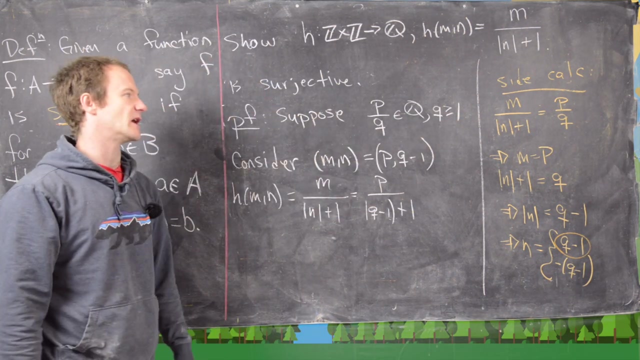 So we know that when we write a rational number as a ratio of integers, this q has to be not equal to 0. But it could be positive or negative. But if it's negative, we could just take that negative and absorb it into the p upstairs, meaning that we can always assume that q is positive. 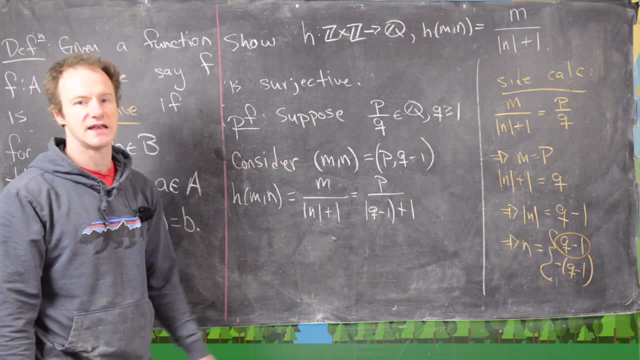 Great. But if q is positive, then q minus 1 is non-negative, which means we can get rid of those absolute value signs, 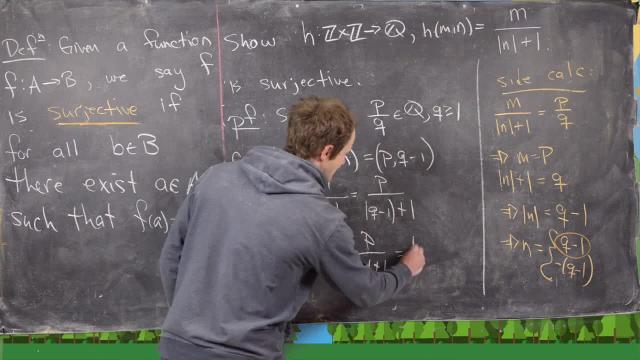 which means we get this as q minus 1 plus 1 or p over q. Great. 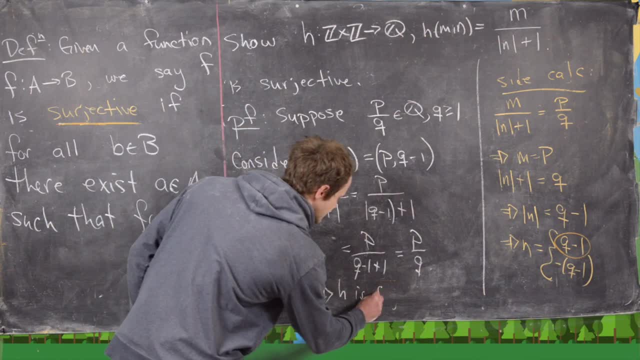 But that's exactly what we need to show that h is surjective. And that finishes our proof. Okay. That's a good place to end this video. 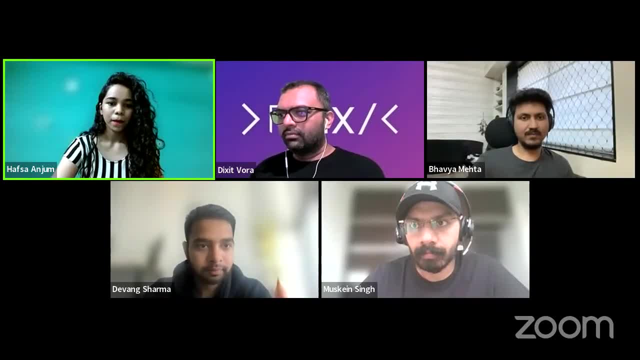 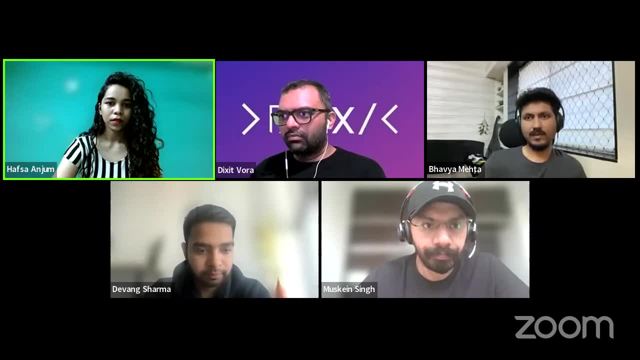 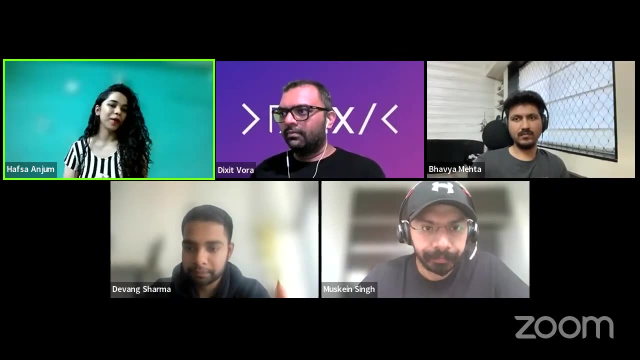 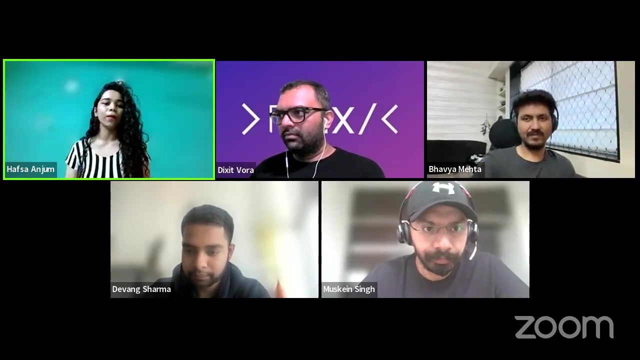 And for people who are joining us on Zoom and LinkedIn and YouTube or anywhere else. if you think that we're live, please make sure that you're introducing yourself in the chat. Let us know what's your name, where you're coming from and what you're working.